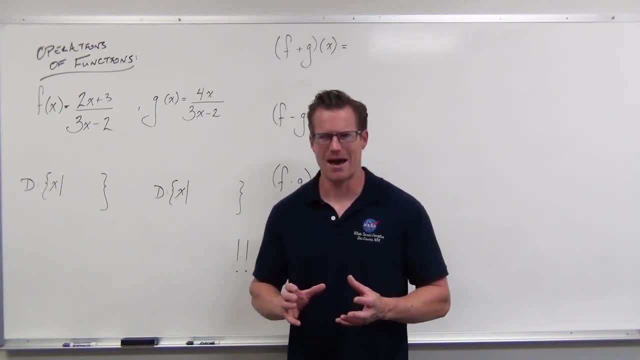 domain. it's one of the most pessimistic attitudes that we have, right? So domain is like the skeletons in the closet: You can't ever get rid of them. They're always there, Like it carries its baggage with it all the time. So when we start to compose functions or add functions, subtract, 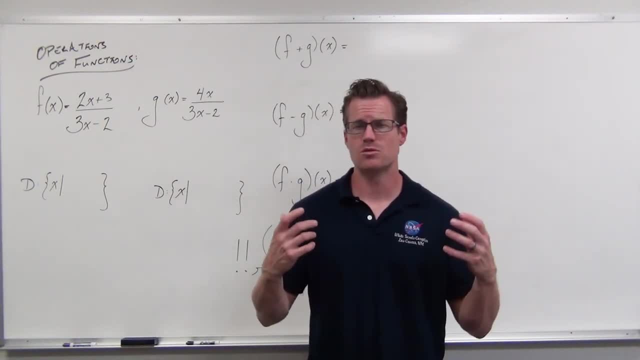 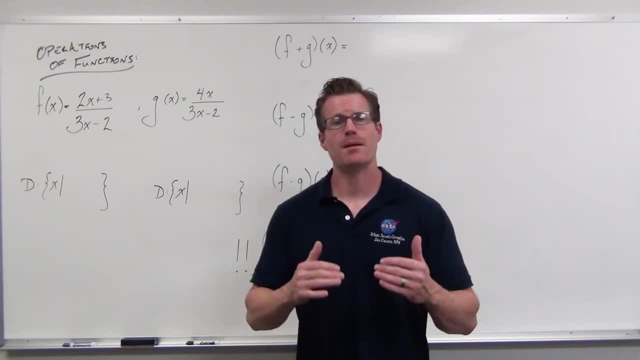 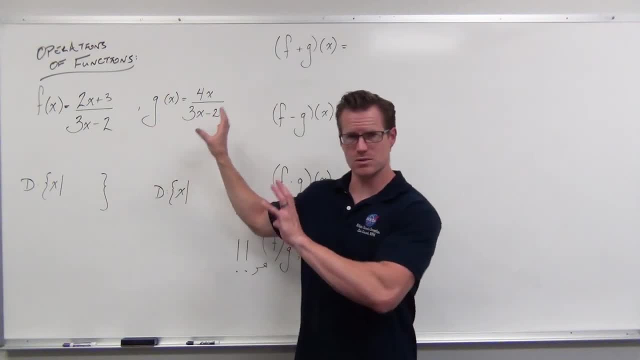 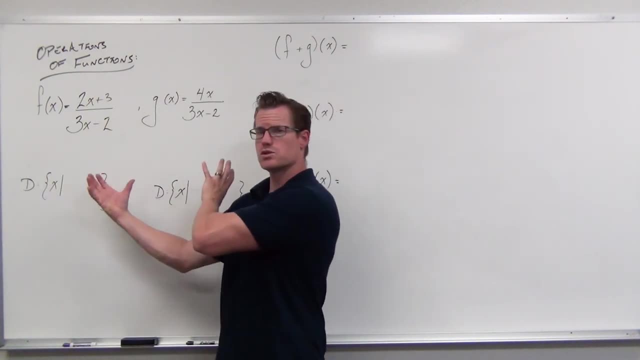 find the domain for each of them. This is very easy because I gave you a nice one. that's the same. And then if we add them, subtract them, multiply them or divide them, we are going to have both of those domain issues in every one of these cases. And then 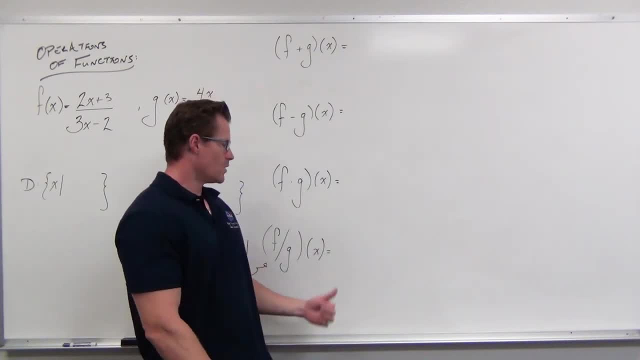 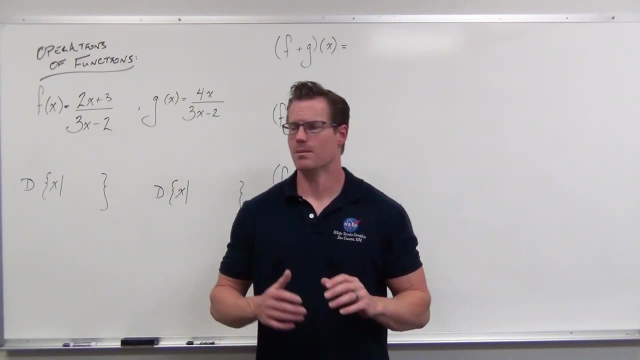 what's even a little bit kind of worse about it is that we can even develop some new domain problems by doing these operations. So that's what we're going to be looking for in this video. I'm going to show you how we can add, subtract, multiply, divide functions. We'll simplify them. 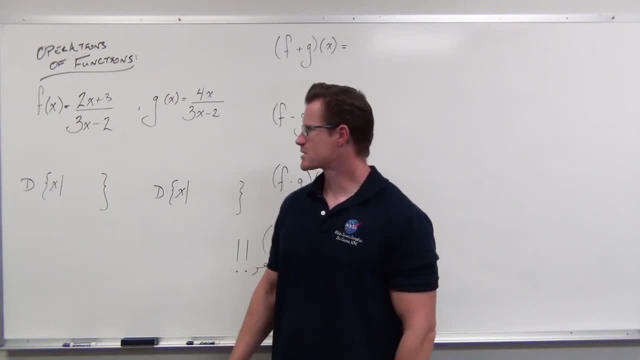 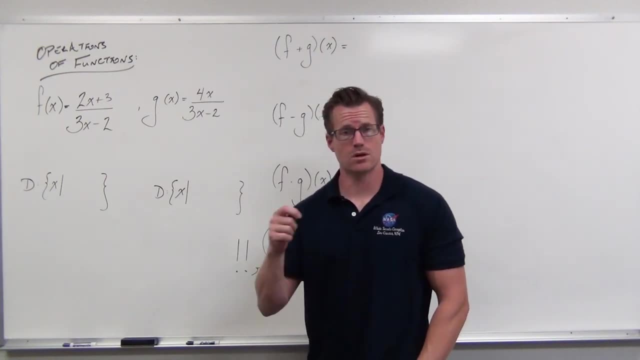 as much as we possibly can, And then we'll discuss the domain. So let's start right now. Whenever you're going to do operations with functions- whether that's going to be addition, subtraction, multiplication, division, or if you're going to start composing functions- 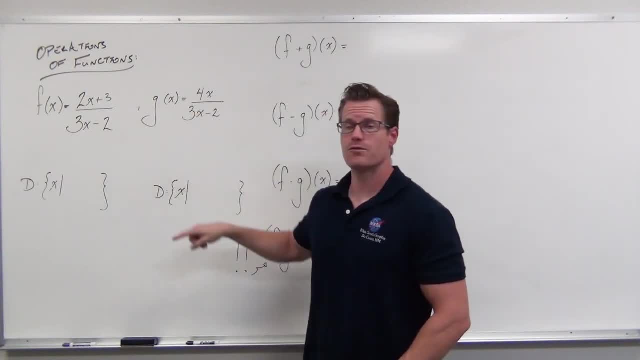 the first step that we do is we find the domain for each of our functions individually. Now here they both got fractions And after watching the last video you know about fractions, you know that we're looking for inputs that give us a real number, defined output. 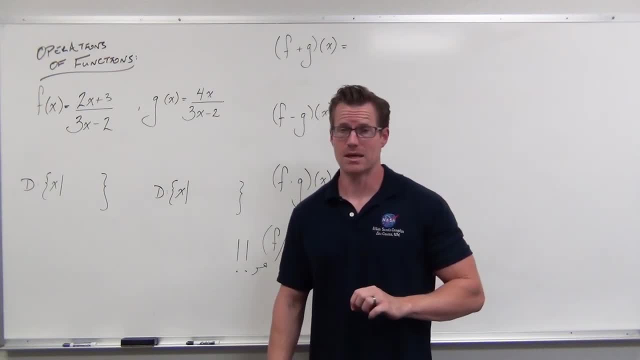 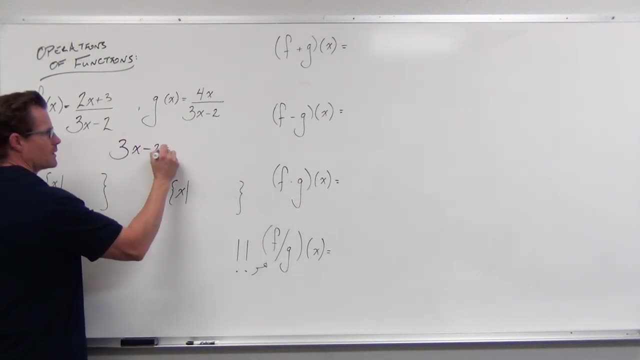 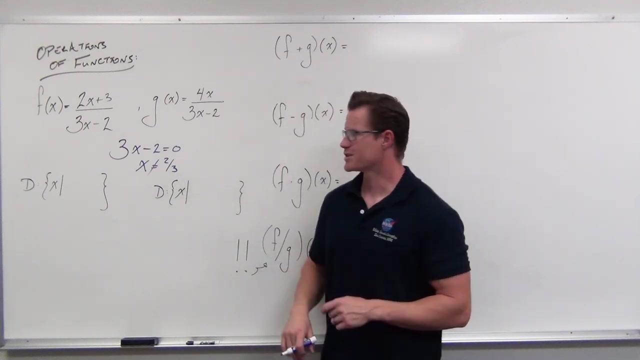 which means for fractions, denominators equaling zero are bad things. We're going to set our denominator equal to zero, understanding that when x equals positive two thirds, that's a problem for us And it's the same problem for both of these fractions I gave. 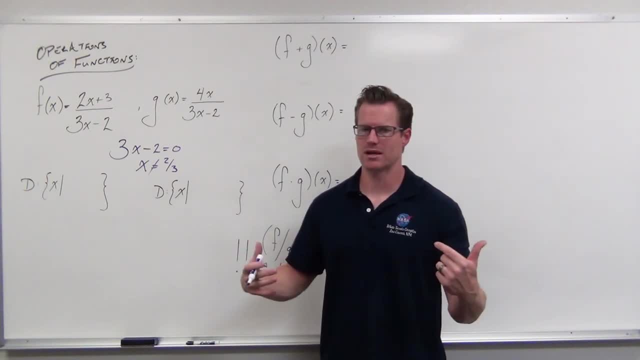 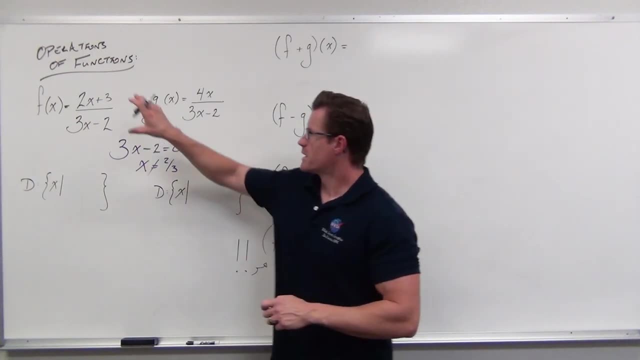 you the fractions, like this, with the same denominator, so that we can add them and subtract them easily. I'm not trying to teach you that. I'm trying to teach you what happens with the domain Here's, especially with this case. So here our domain says: you're good as long as x cannot equal. 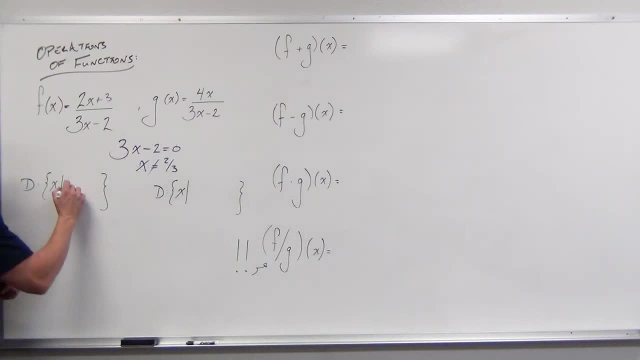 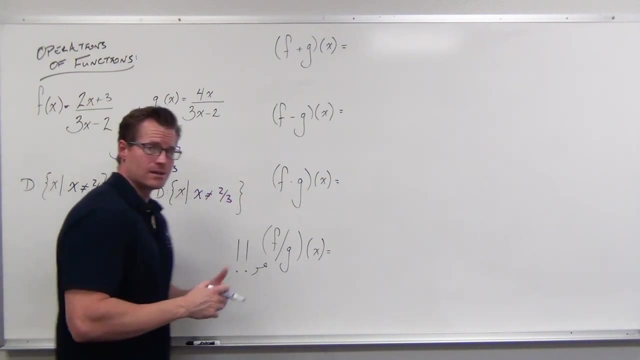 two thirds. And sometimes we even abbreviate that and say: hey, x such that x does not equal two thirds, x such that x does not equal two thirds, implying that all real numbers work except for two thirds, because that would make my denominator equal to zero And that creates an undefined 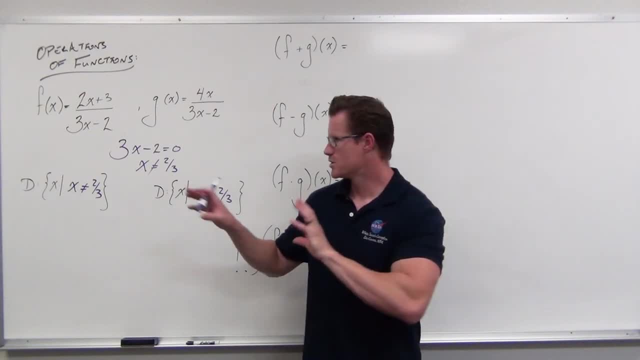 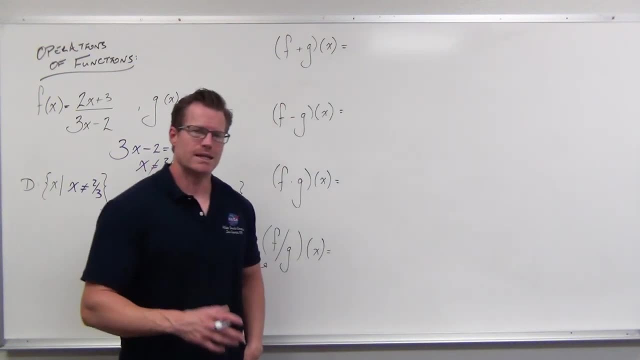 result for that particular input. So that's got to make sense. Two thirds as an input don't work because your output is undefined. Now, when we start adding functions together, I need you to remember, I need you to know that, no matter what we get, 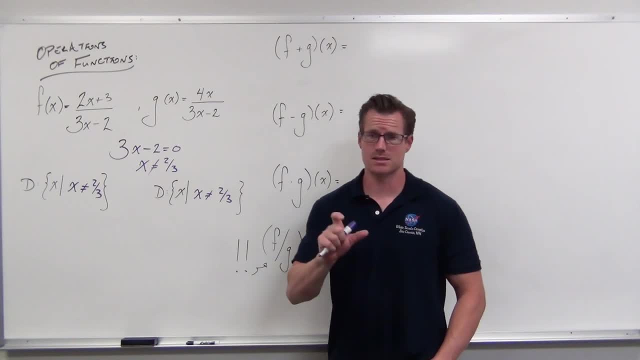 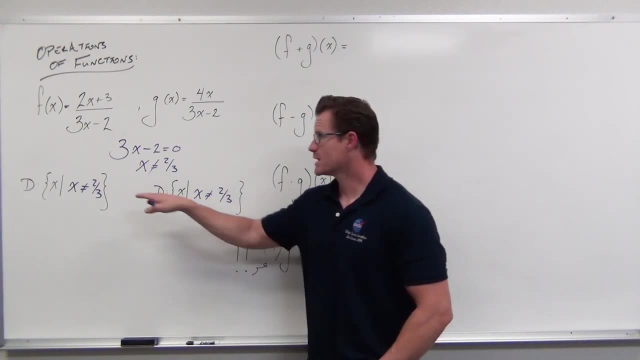 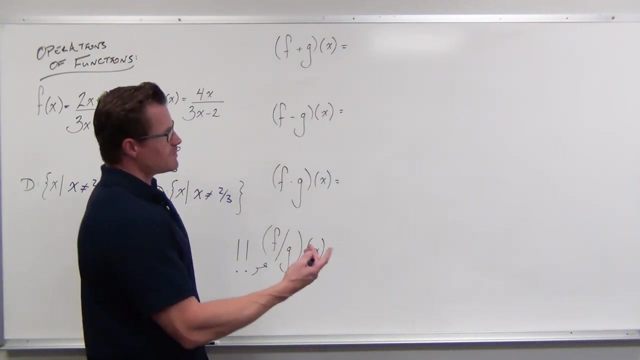 this right here is going to be the domain- at least this right here is going to be in the domain- of the resultant function. we could get worse things from it, but we can't ever get rid of these problems. They stick with your functions forever, no matter what you get Now, typically with addition, subtraction and multiplication- 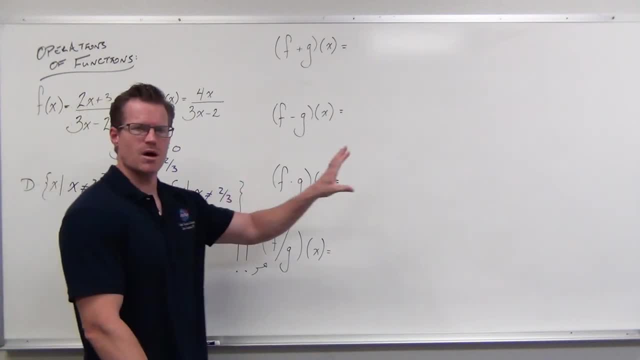 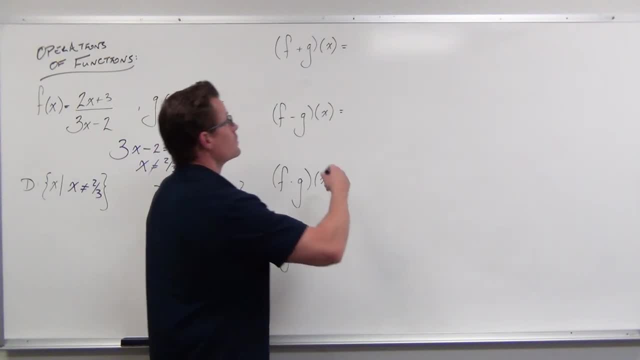 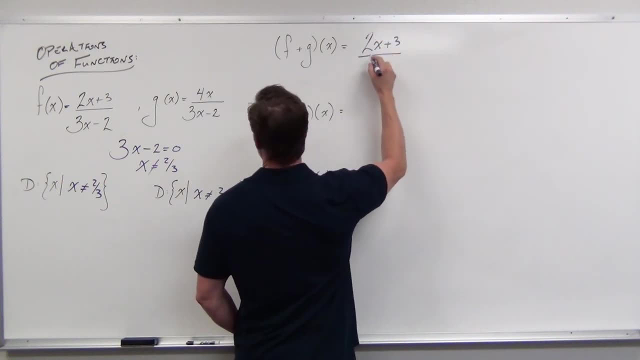 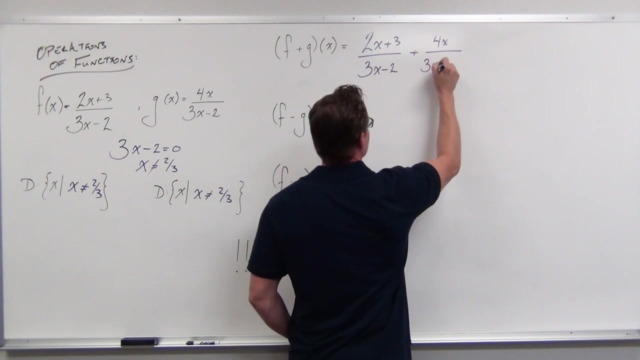 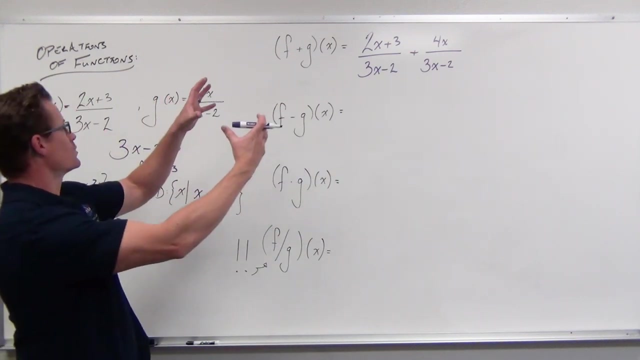 deal for those, but for this one it is, and we'll see why in a minute. So f plus g of x. if we add these functions together, keep in mind that we need a common denominator to add fractions, and we have that, so we're just combining the numerators. 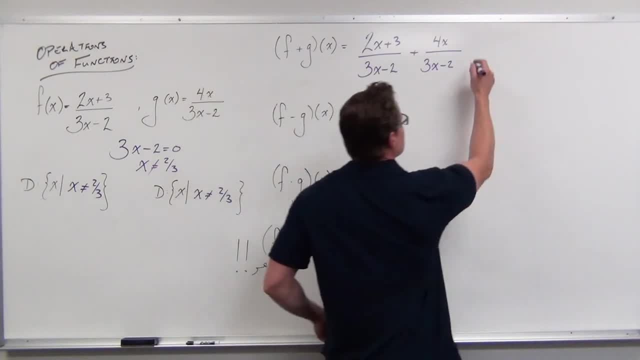 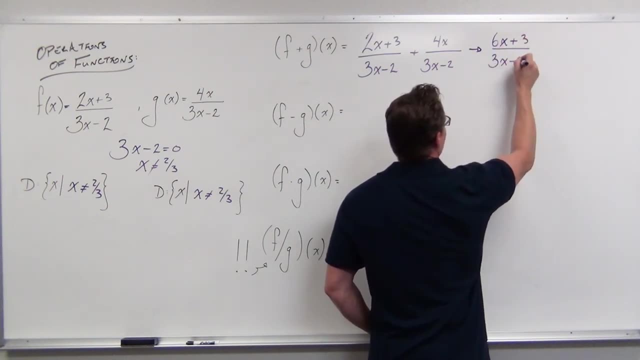 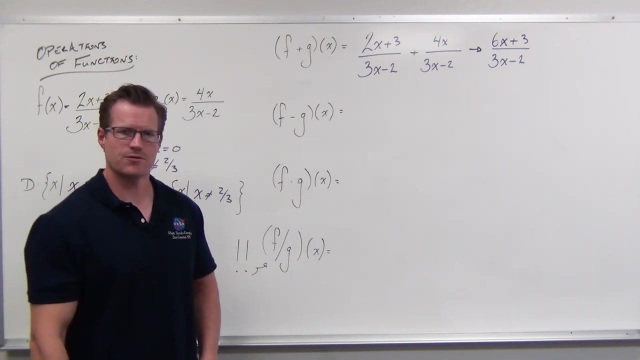 right now That looks like 6x plus 3 over 3x minus 2.. Yeah, you can factor the numerator, but it's not going to help you simplify, so I would leave it just like that, because if we ever have to deal with it later, the first thing we're 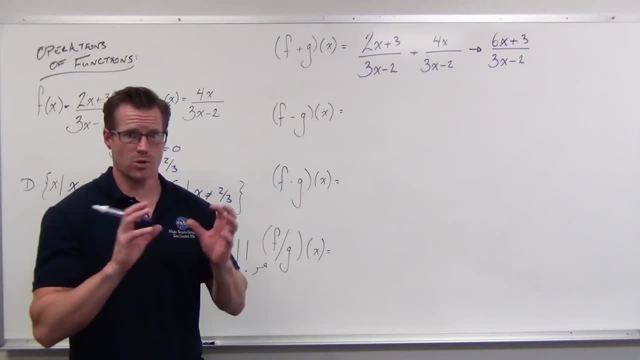 going to do is probably distribute that numerator. Denominators should always be factored, so, if not, you should factor that. Now, here we can't do it, but that's something to think about. Okay, so we're going to do that. So we're going to do that. So we're going to do that. 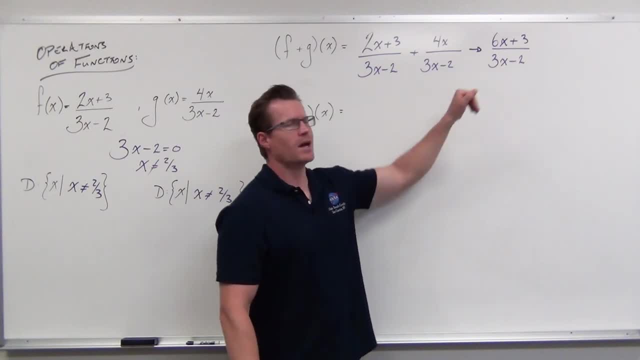 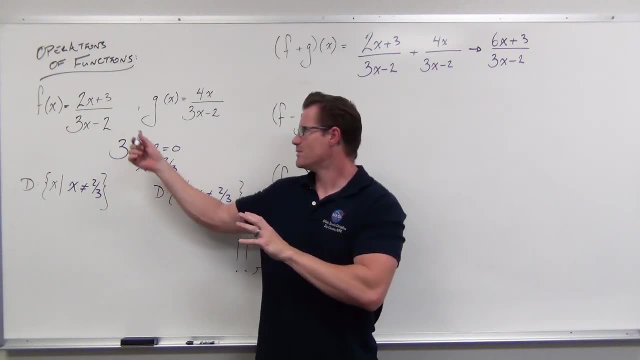 And notice something: Your resulted function here has the same exact denominator, obviously, as what we started with. That means that your domain is going to be the same. Even if these denominators had been different, you would have found a common denominator, wouldn't you? Which means you'd have the 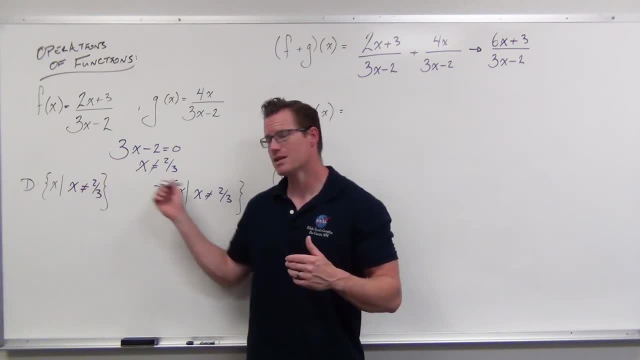 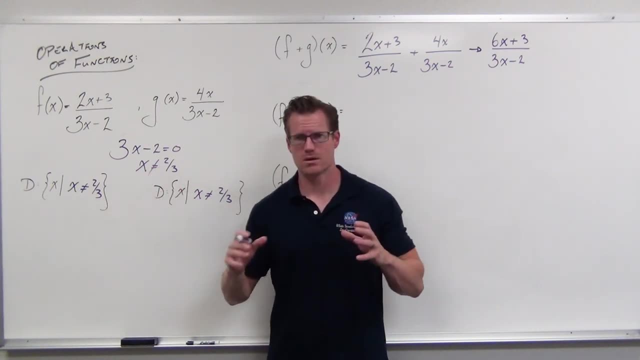 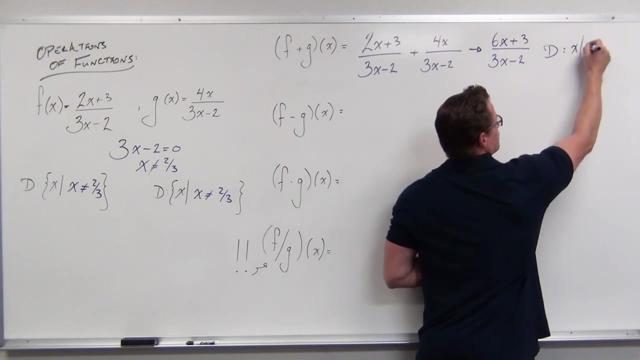 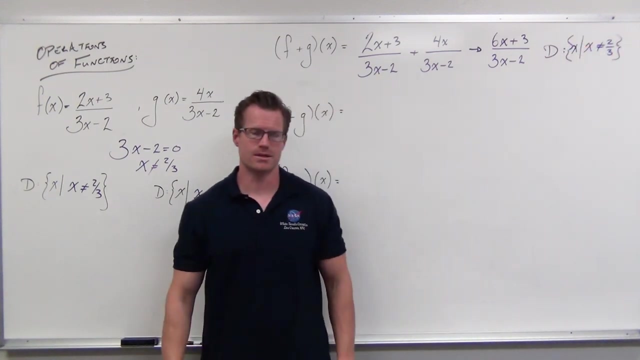 same factors, and those factors equaling zero would cause domain issues for you. So even if your denominators are different, you'd find a common denominator and these things would appear again, whatever they are, in that result. So our domain says: hey, I'm going to be exactly like how you started. 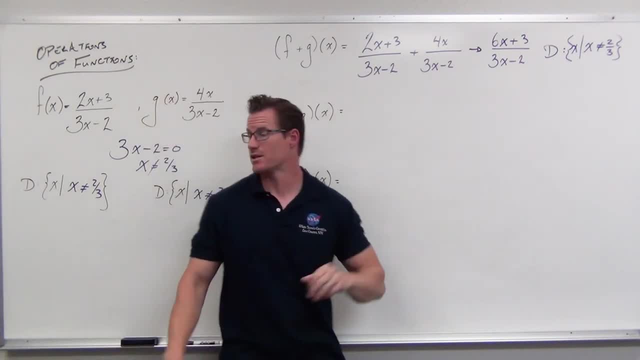 The same thing's going to say: sorry, I'm going to be exactly the same domain as what you started with for both of your functions combined. whatever those are Here, they were the same. They don't have to be, They'd just be different. 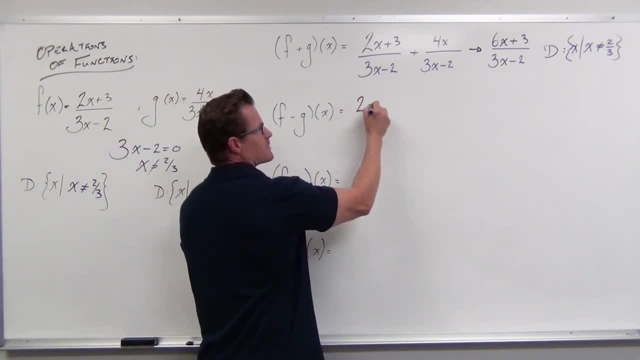 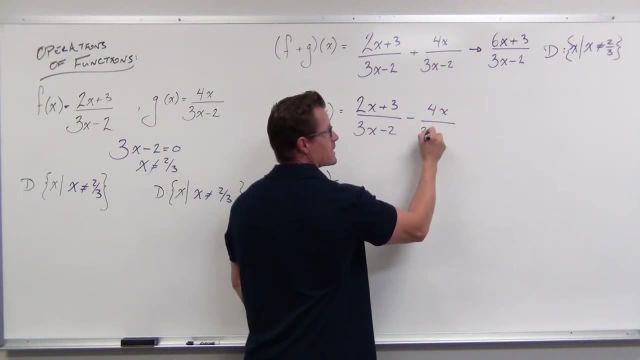 denominators f minus g of x is identical, except that we're subtracting. but we're also going to see that when we subtract that 4x over 3x minus 2, I have a 2x minus a 4.. 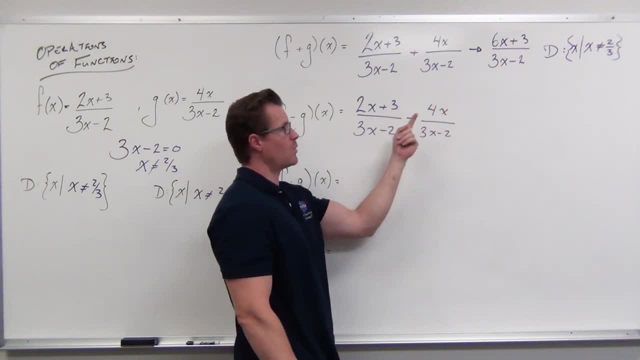 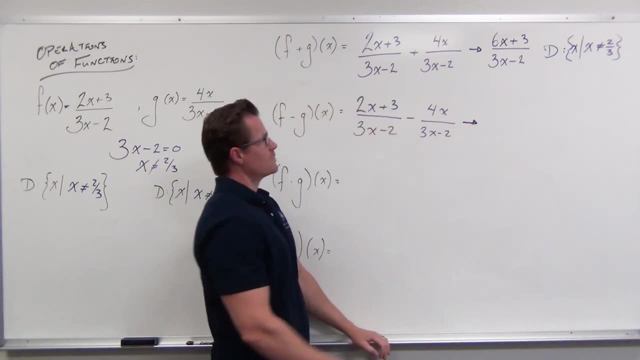 Keep in mind if this had more than one term. I want to show parentheses. I want to distribute that minus because you'd be subtracting every part of that numerator and we should know that. So minus 2x or negative 2x, plus 3 over 3x. 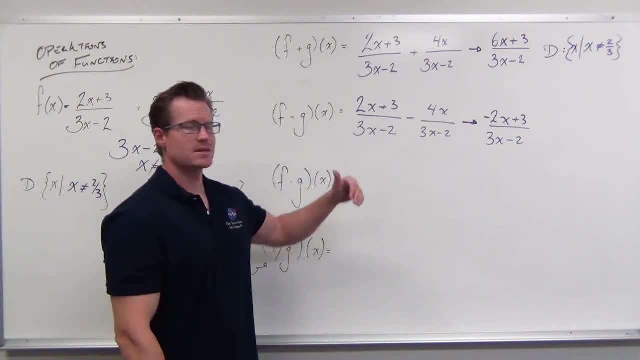 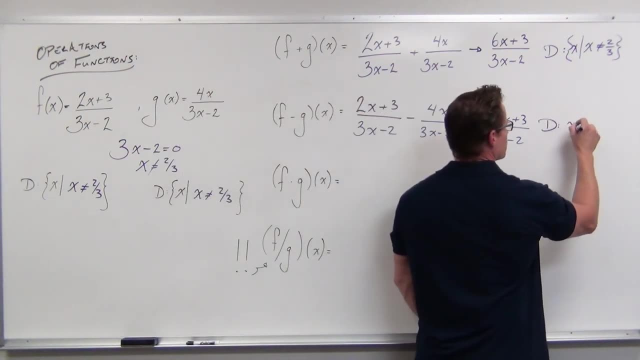 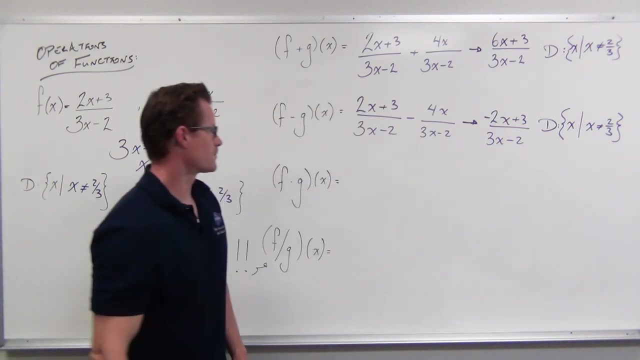 minus 2.. Again, there's no simplification that we do and we see that the domain that we had originally is going to be the same domain that we give to that when we subtract functions. You know what, if you think about it with multiplication. 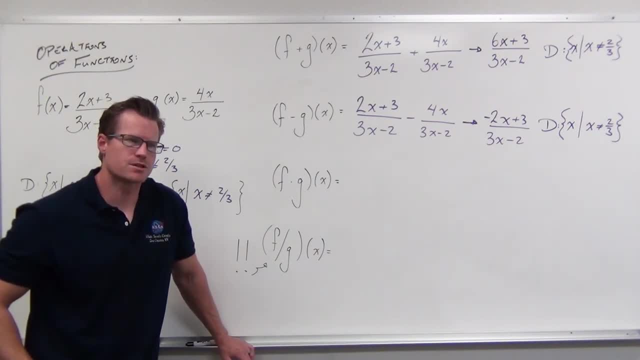 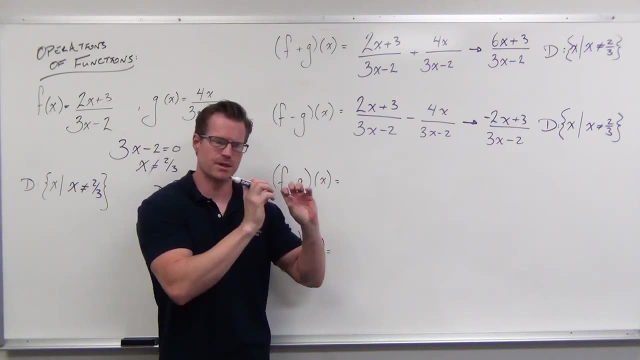 think about what happens when you multiply fractions. Well, you take the denominators and you multiply them together and they they basically become the new denominator for your fraction. Now, if we simplify stuff, we can accidentally start simplifying away one of those domain problems. But if you 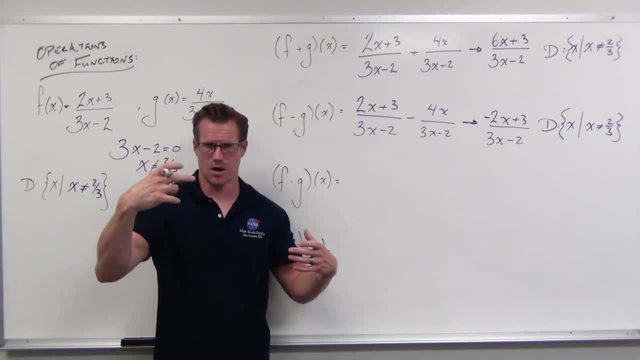 think about what happens in the domain. I'm going to have one fraction with the problem of the denominator and another fraction in general problem of the denominator. I'm going to multiply them. that becomes my new denominator. Do you see how I'm just going to keep combining my domain problems for addition and for. 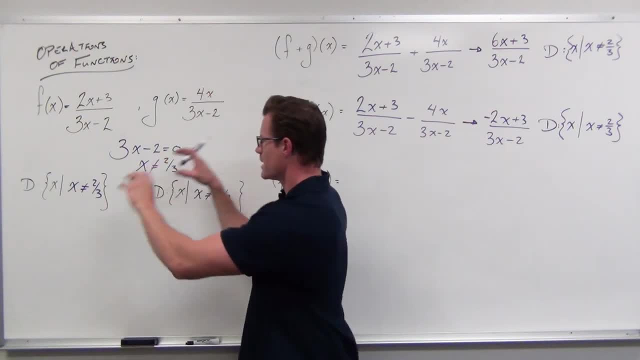 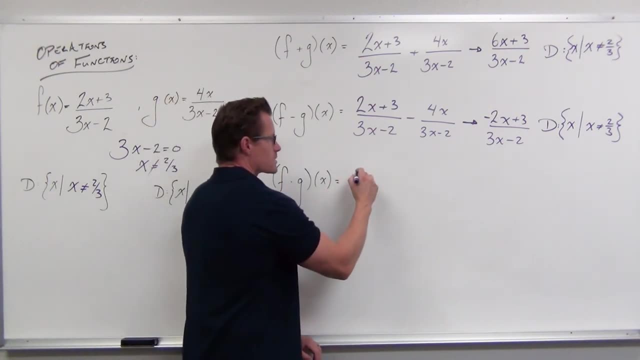 subtraction and even for multiplication. We're going to get the same domain here moved over to this. That's going to be the same domain, as what our result is is what we we started with. So this 2x plus 3 over 3x. 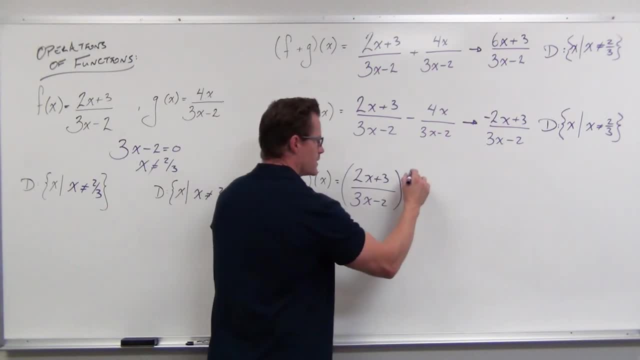 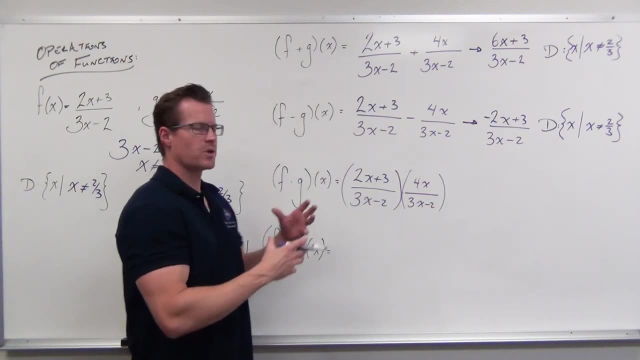 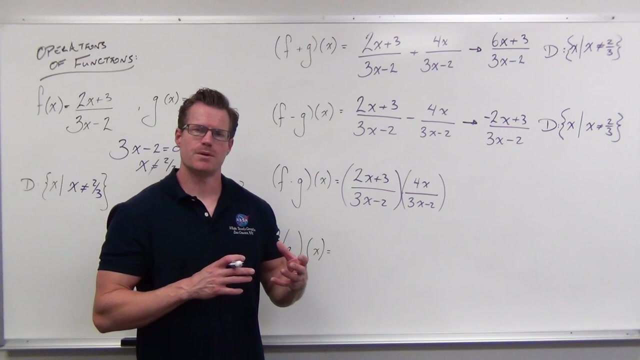 minus 2. probably parentheses would be good here. Multiplying fractions says: multiply your numerators. we're going to distribute the 4x. Multiply your denominators, we're not going to distribute at all. Your denominators should always be factored as much as possible, So instead, 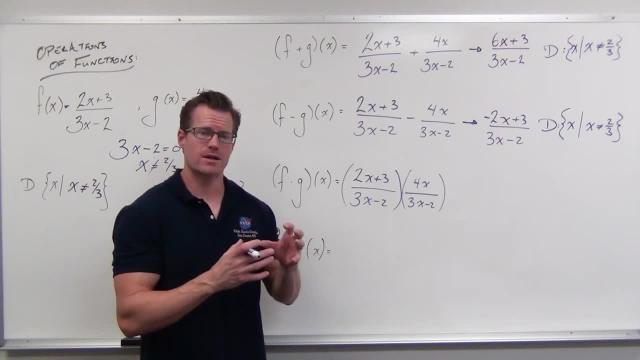 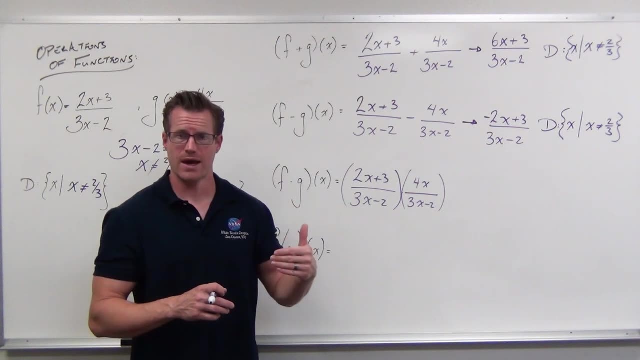 of distributing 3x minus 2 times 3x minus 2. we leave them factored for a variety of reasons. One of them is because when we graph these things, it's really nice and very appropriate to have your denominator factored. It would. 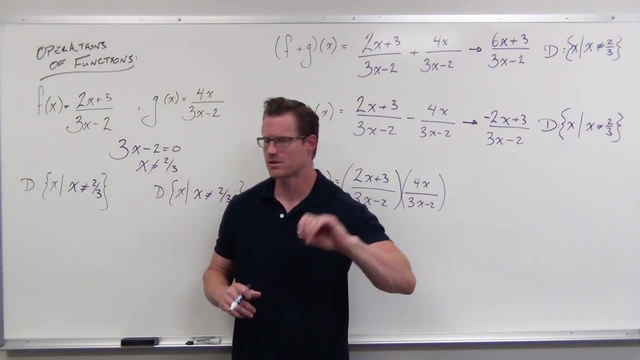 create a vertical asymptote. We haven't got there yet, but I said that in the last video. It created a vertical asymptote at 2, 2 thirds. at x equals 2 thirds. This is this kind of force field you can't touch. 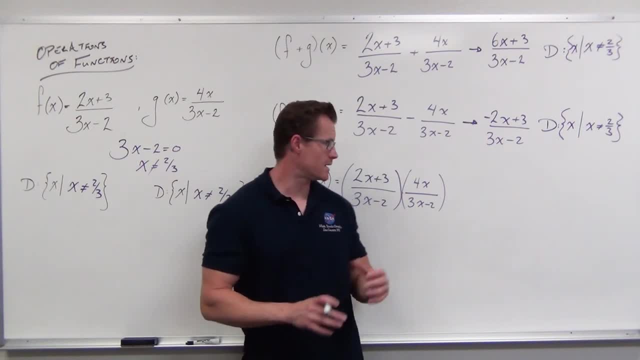 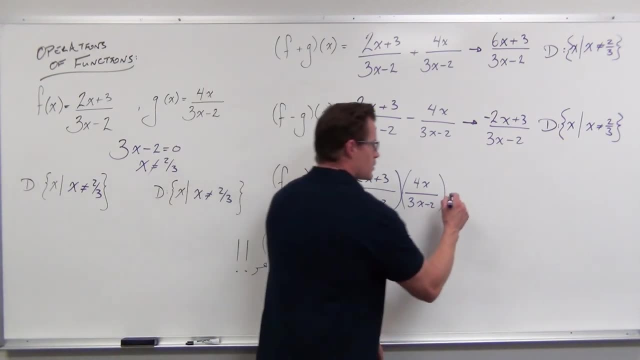 And then, because that powers there, because we're going to have this group as 3x minus 2 to the second power, it's going to tell us a multiplicity of that. We're going to get to multiplicity later, So we'll distribute numerators, Absolutely So. 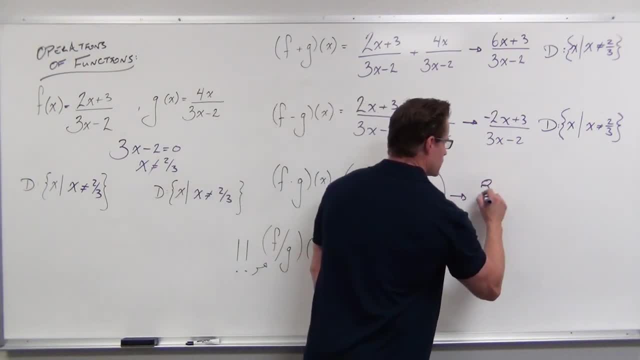 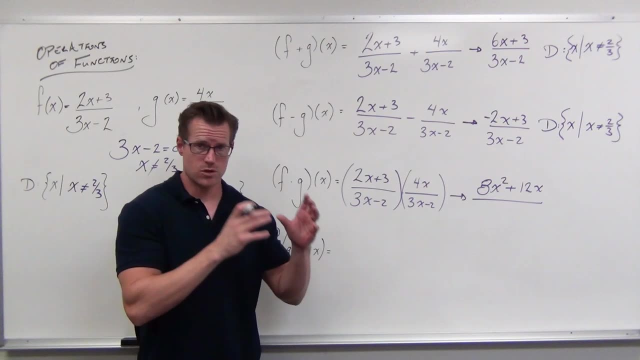 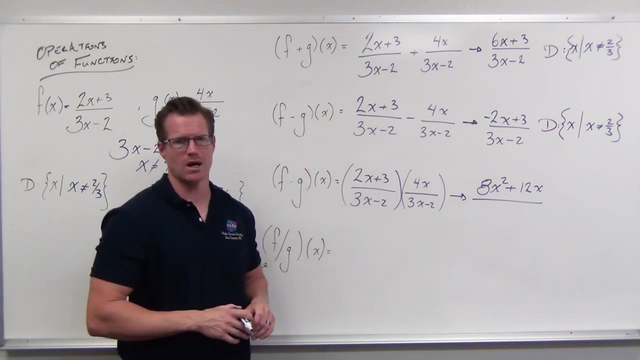 that's going to be 8x squared plus 12x on the denominator. Leave your denominator factored, So I don't care what these things are, whether they're the same or not. You leave them as factors. It's going to really help you with graphing, I promise. And if we ever have to add fractions or simplify, 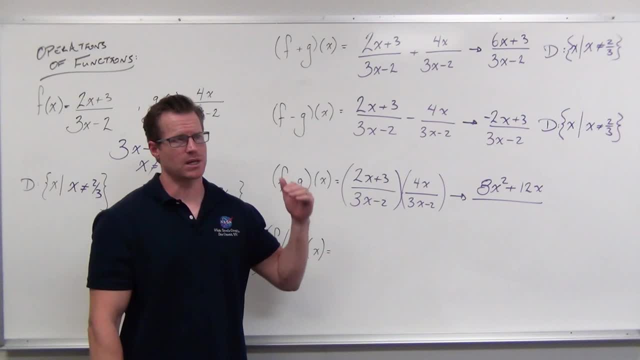 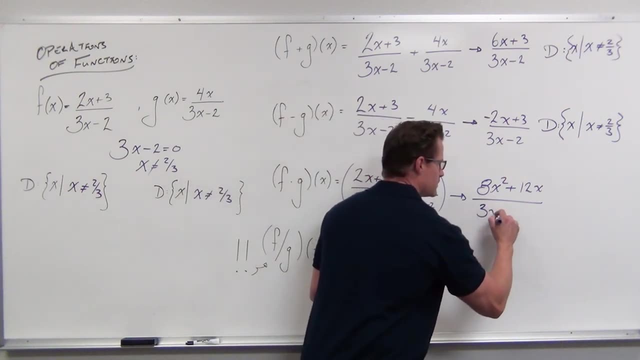 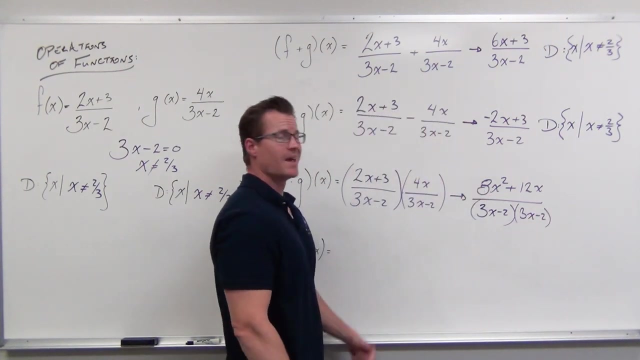 fractions or multiply them. we can find LCD easier, We can cancel out, simplify easier, We can do everything easier. if we leave these factored Now, because we have 3x minus 2 times 3x minus 2, that's a repeated factor, That's repeated multiplication, That's an exponent. 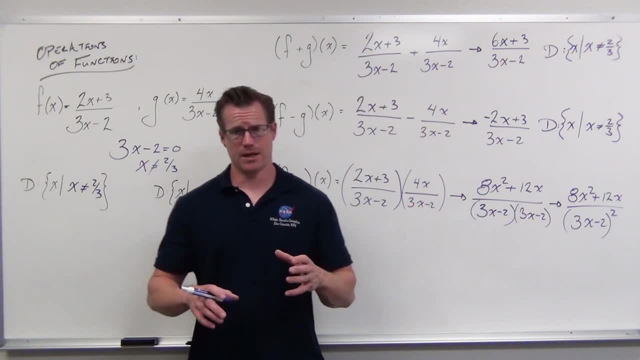 So that's a repeated multiplication, That's a repeated multiplication, That's a repeated multiplication. That's how I want to see it. And do you see that, no matter what, because you're going to keep these factored, you're going to see the same exact denominators that you had here. So the same. 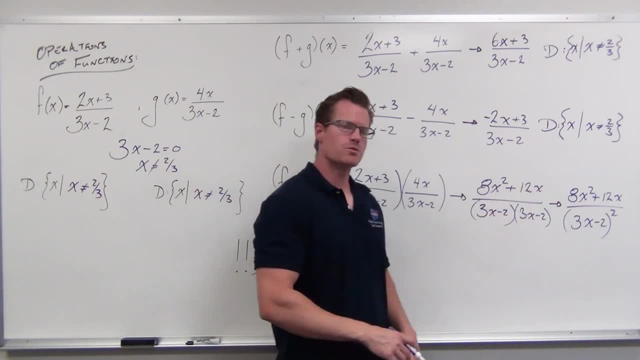 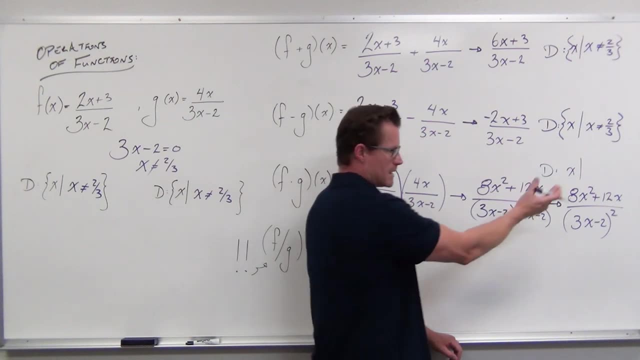 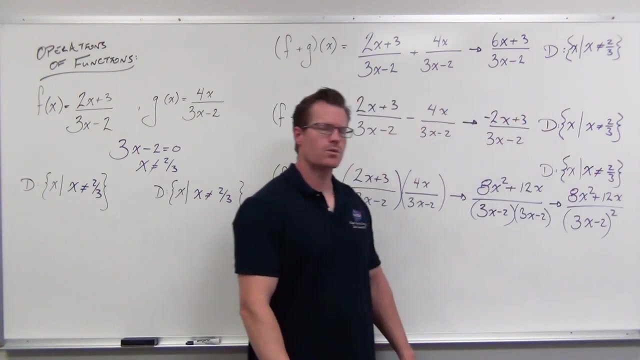 exact domain issues that you had here. those are going to repeat over here, So our domain doesn't change. Our domain says: yeah, your domain for this is x is such that x cannot equal again two-thirds. I want to reiterate this. I know that I haven't taught it to you. 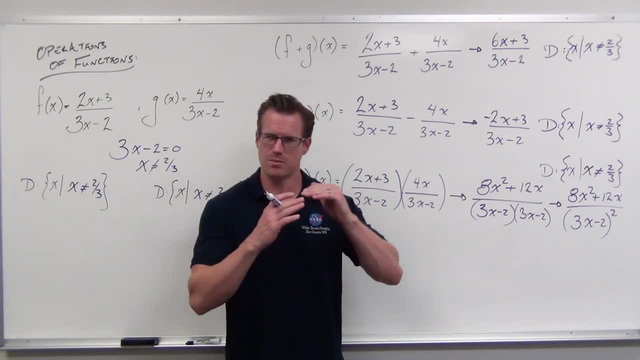 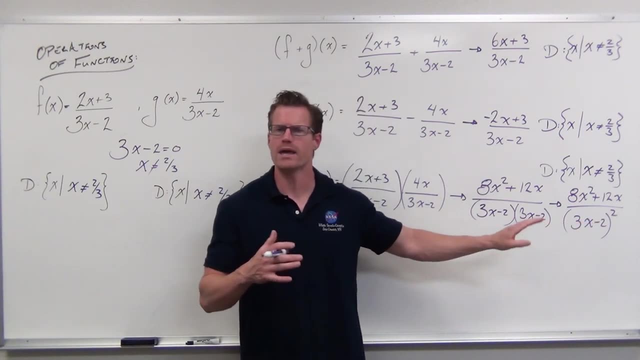 yet. but you know how I teach. at this point, You know that what I'm trying to do is prepare your brains. I'm giving you an advanced organizer for later on as to why you do this. Sometimes, if you don't know why you do something, it's really hard to accept that you have to. We have to do this, and 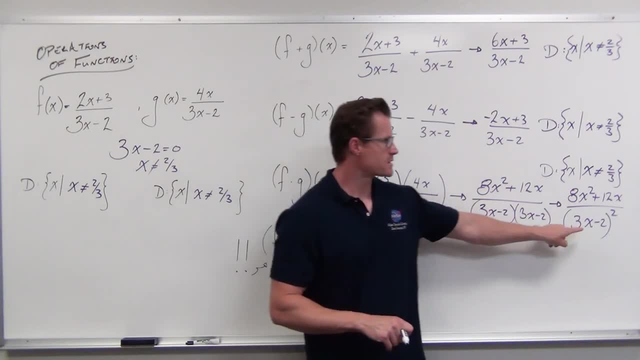 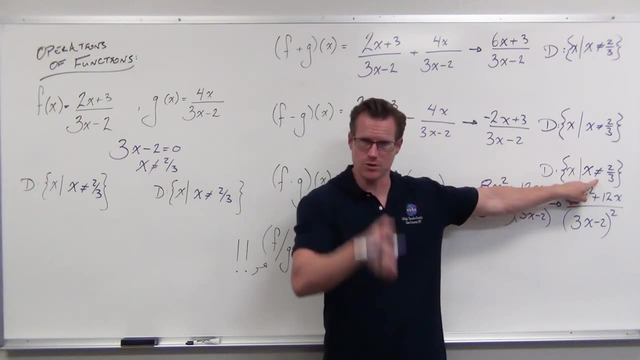 leave it factored and write the exponent, because later on this is going to give us a vertical asymptote on a graph at that value. So a vertical line- x equals a number- is a vertical line. If x can't touch, can you Do, you, Don't you? Can you One of those? You have something that you can't. 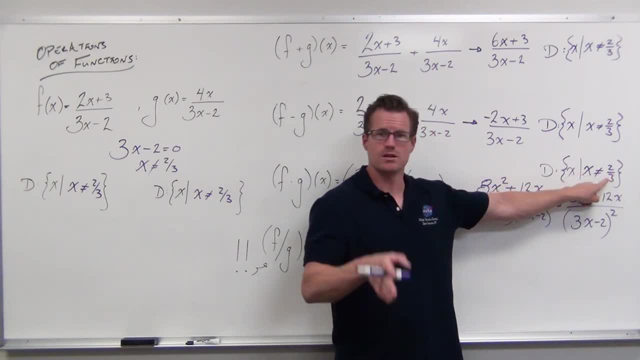 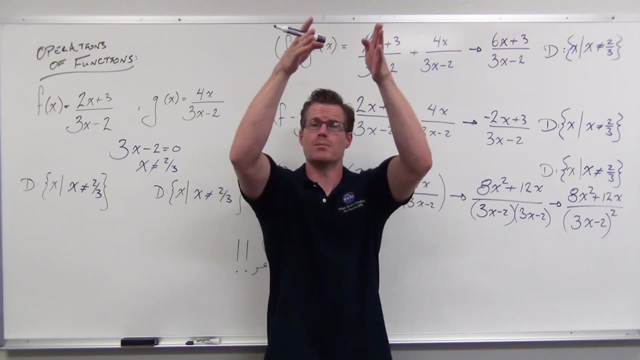 touch, don't you? Well, if you have something you can't touch, then you have a vertical asymptote and that power says that you're going to be even. Even functions match up. So we're going to look like this or look like this around the asymptote. That's why we leave it that way. I'm going to. 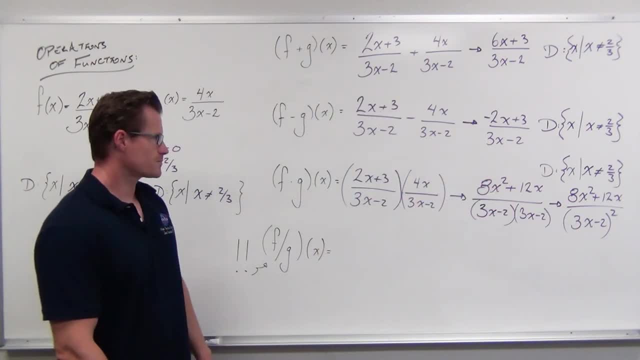 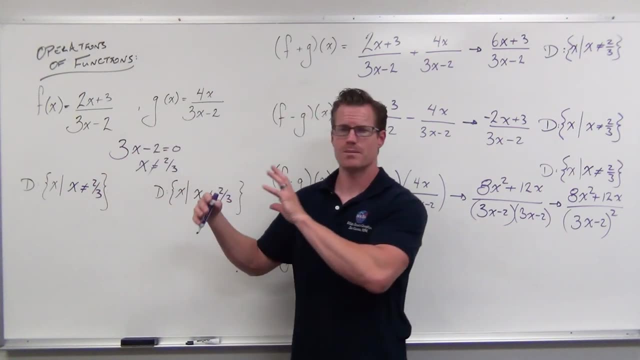 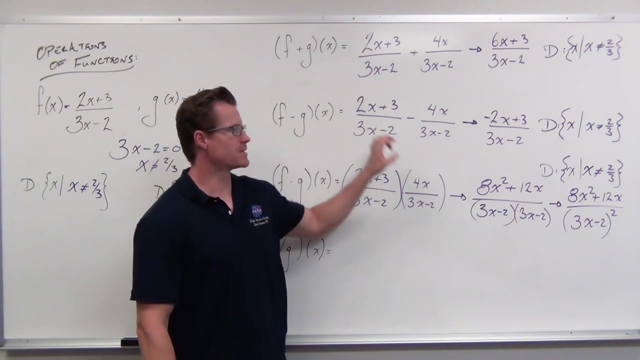 flesh that out in a few more videos. So long story as short as I can make it. domain is still really relevant for your functions. We talk about it lots and lots moving forward. Find your domain first. If you have to add subtract or multiply functions, you're going to get the same domain. 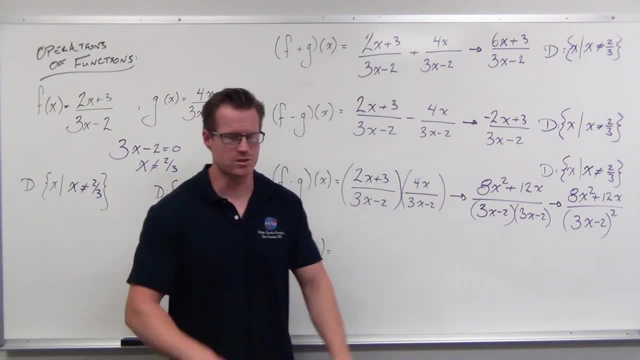 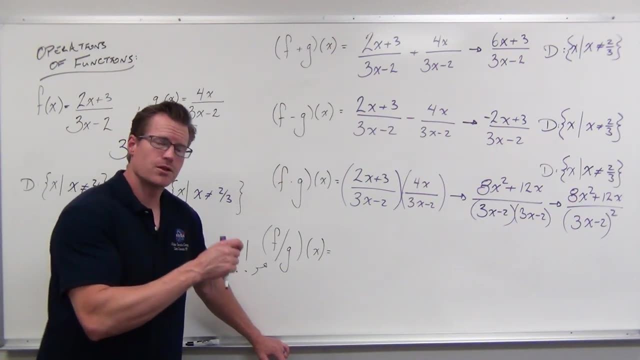 almost exclusively. There are times when you don't, but almost exclusively you get that If you divide, not only are you going to get the same domain, you could add some other issues to that domain- the domain problems you already have. The key here, though, is that when you 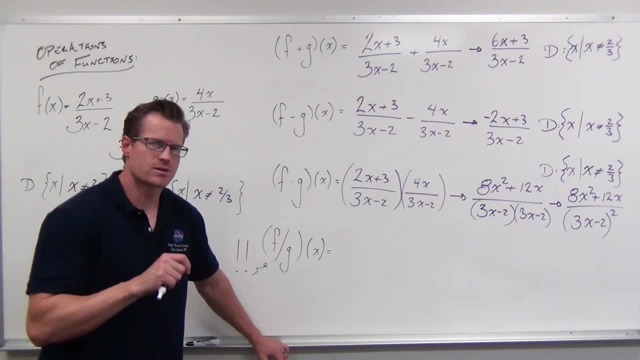 start dividing. it's going to look like you can cancel out some stuff. it's going to look like your domain doesn't have a problem anymore. You still have the problem, It's just hidden. So I said this at the beginning and it's going to make some sense as we go through. 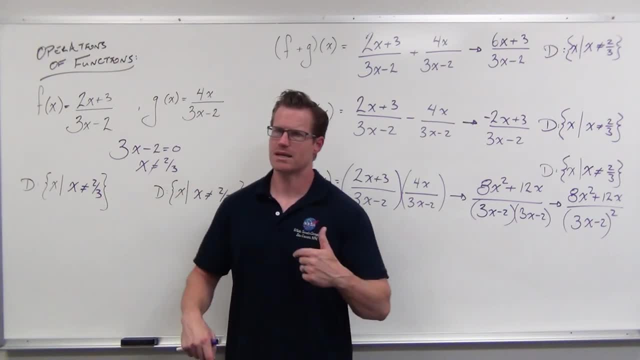 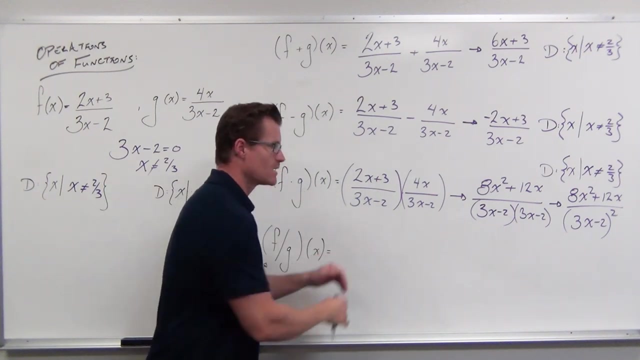 but these issues, this x can't equal two-thirds that issue because the resultant function starts here. It is these things just wrapped up together, Because these are those root, if you will functions, you can't have that two-thirds, No matter what we get here. I can promise you that. 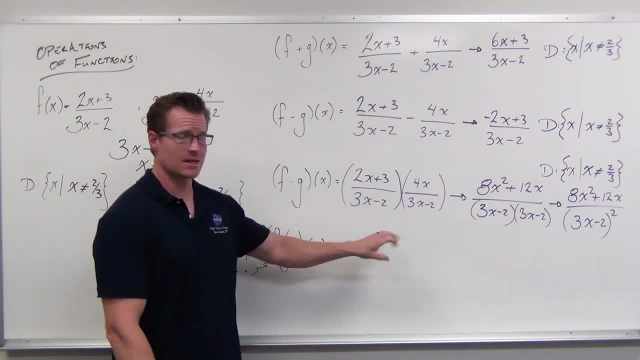 our domain is going to be the same. It's going to look like your domain doesn't have a problem anymore. It's just hidden. So I said this at the beginning and it's going to make some sense as we go through is going to exclude two-thirds from it. It's not going to look that way. It's going to look like we. 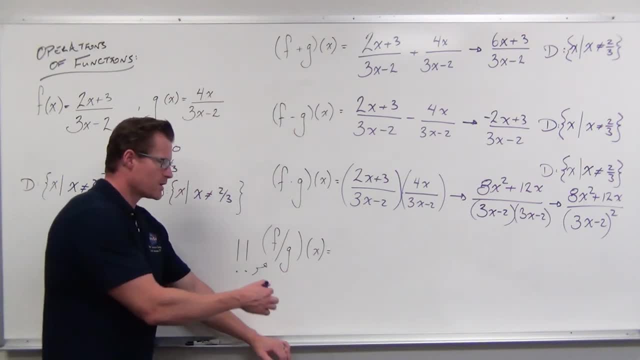 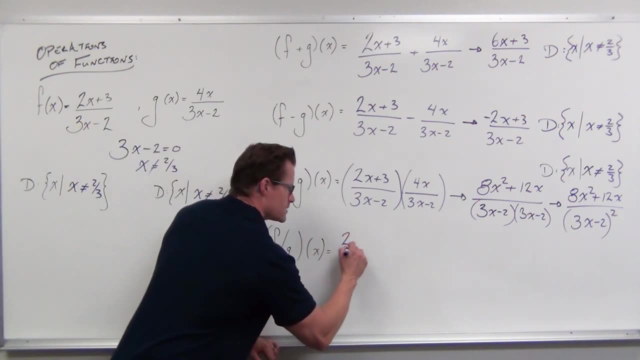 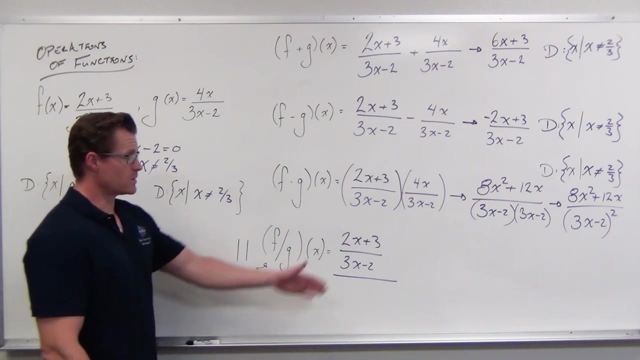 cancel it out, but it still has to be there. So when we divide functions we're really conscious of what goes on the numerator and what goes on the denominator. It says f divided by g. So f is this: 2x plus 3 over 3x minus 2, divided by. you can even write a divided by sign if you want to. 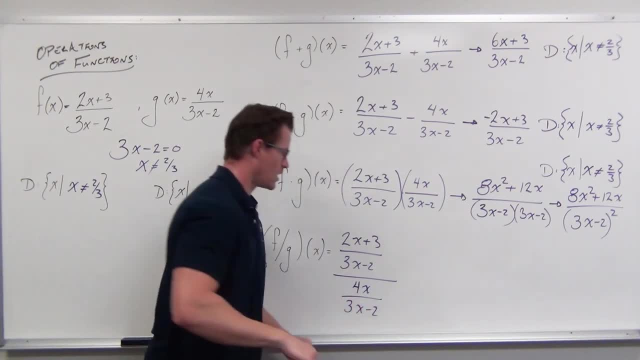 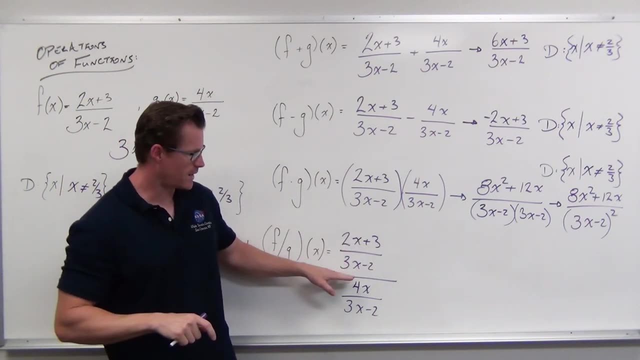 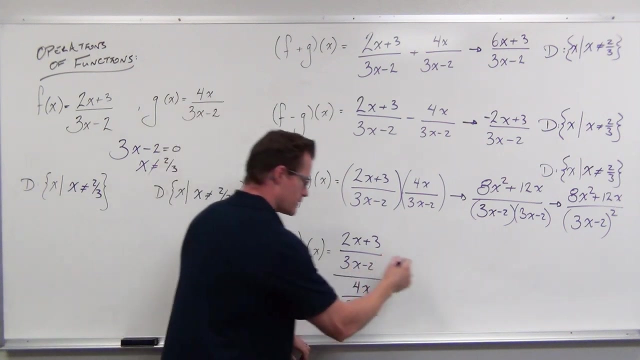 4x over 3x minus 2.. Now we know something about complex fractions. We know that fraction divided by fraction, when we divide, so, fraction divided by fraction, when we divide fractions, we can reciprocate and multiply. So instead of this, we'll reciprocate the second. 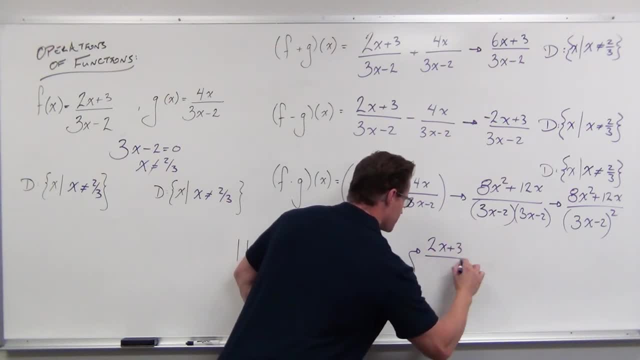 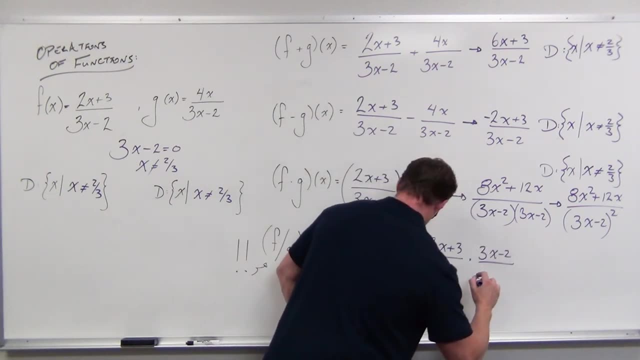 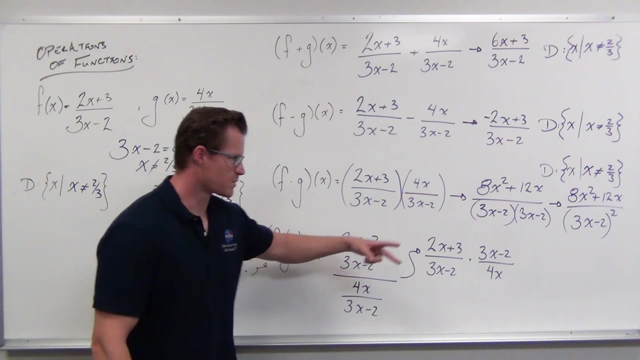 fraction, or the bottom fraction in this case. All right, so I have my first fraction. a problem Division says multiply by the reciprocal of the second fraction And you go wait a minute. Oh, this is awesome because, look boom, Oh, I can cancel out my denominator. I can. 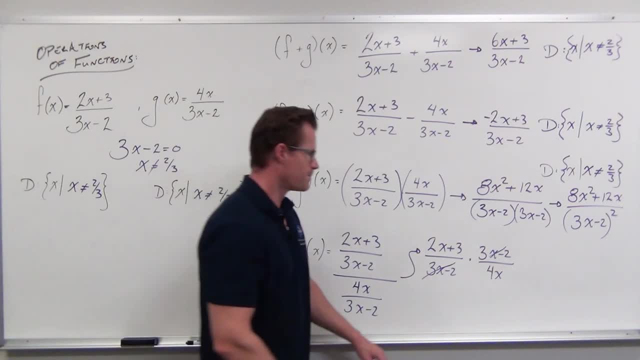 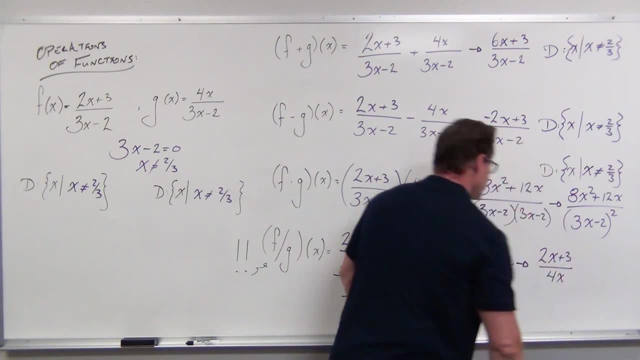 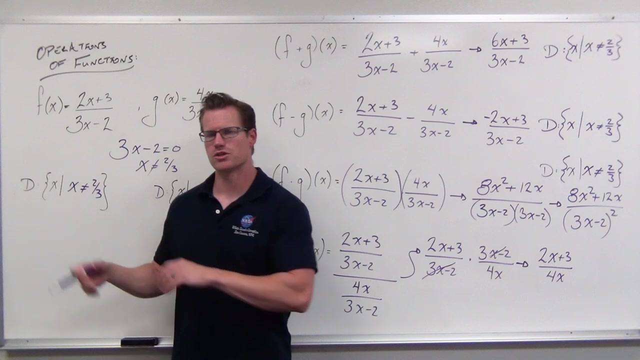 cancel out one of those domain problems. It certainly looks that way. It certainly looks that way, But because of where this came from? because your original functions had a domain of negative of 2x over 3x minus 2, divided by the reciprocal of the second fraction. 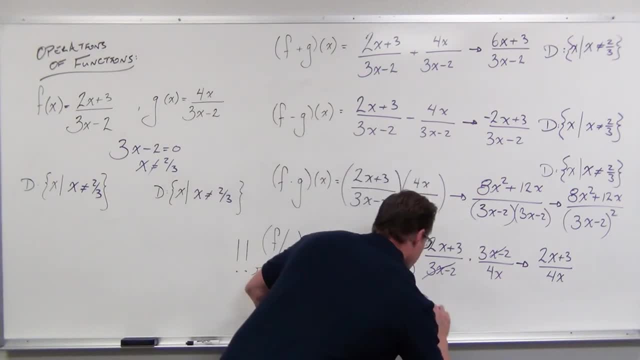 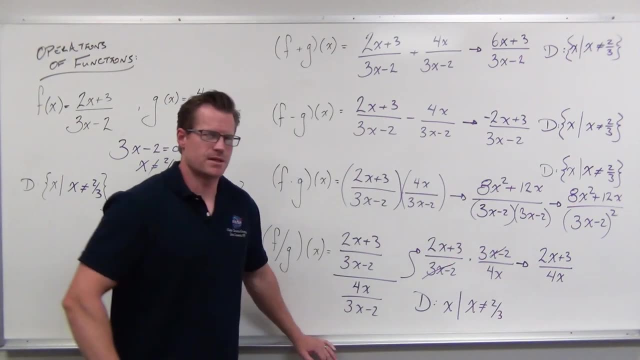 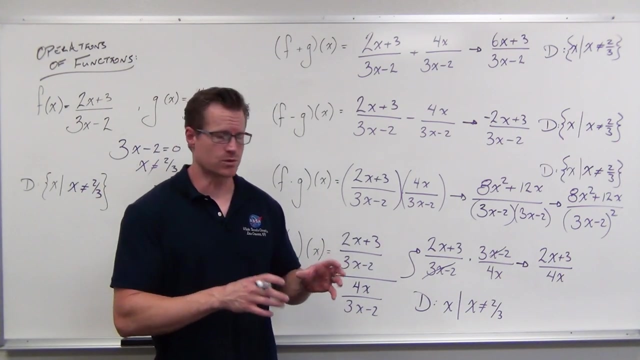 2 thirds is a bad number, so x cannot equal 2 thirds. We actually write that down first, We go through this and go: all right, I know x can't equal 2 thirds and no matter what happens, x cannot equal 2 thirds, Even if I start cancelling stuff out. 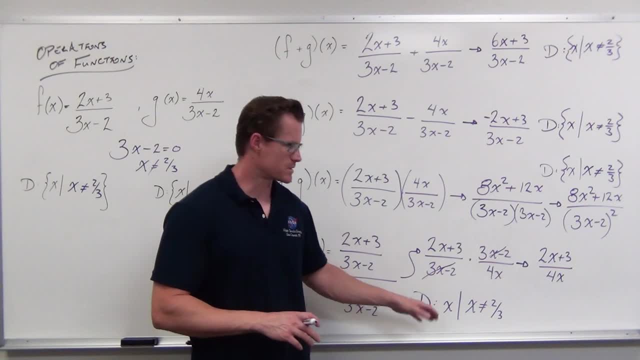 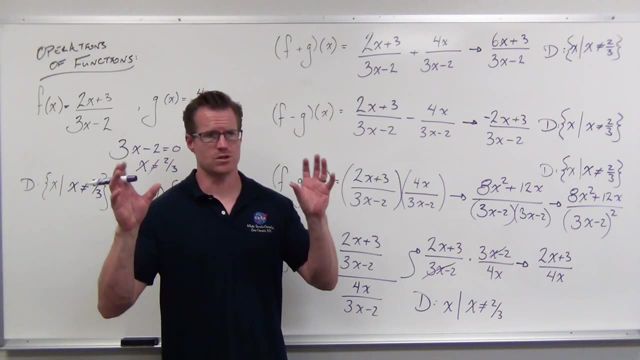 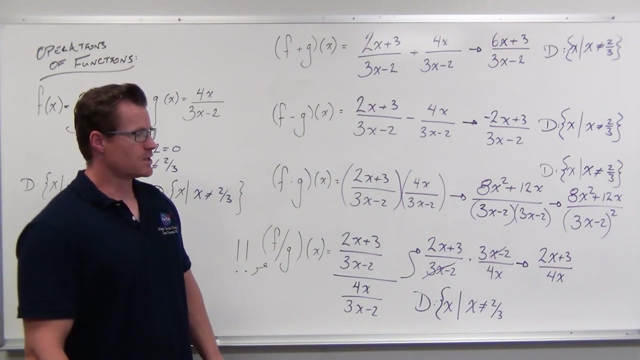 I know that where it came from the baggage it holds onto the skeleton in the closet that you can't see anymore is you cannot allow this function to equal 2 thirds based on those root functions. The other good news here is that you can add some problems to it. So notice our resultant. 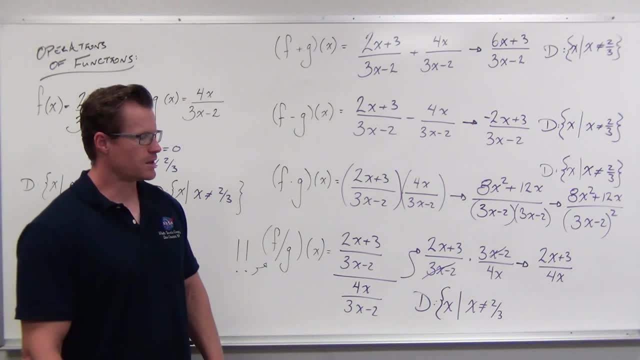 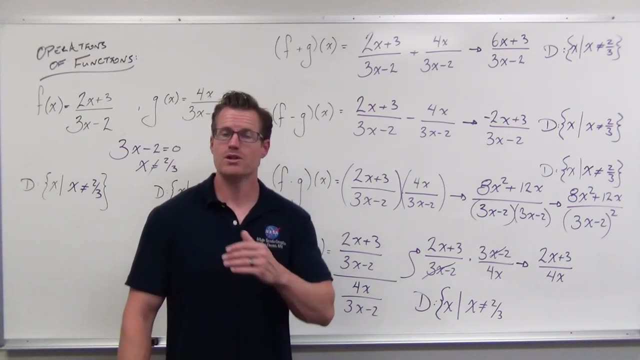 function that we have that 2x plus 3 over 4x And you think about it, you go wait a minute. Wait, that's a fraction with a different denominator than I started with. Yeah, And we know that denominators equaling zero are bad things. So if we continue to go, all right. 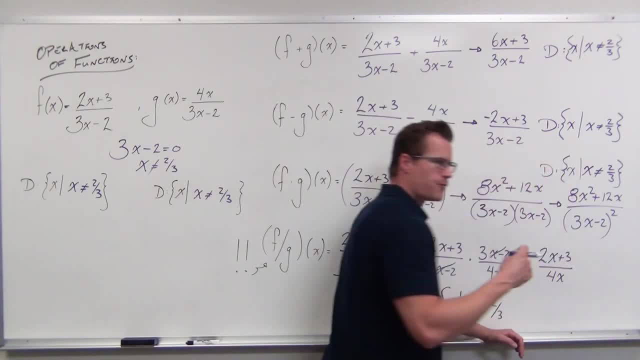 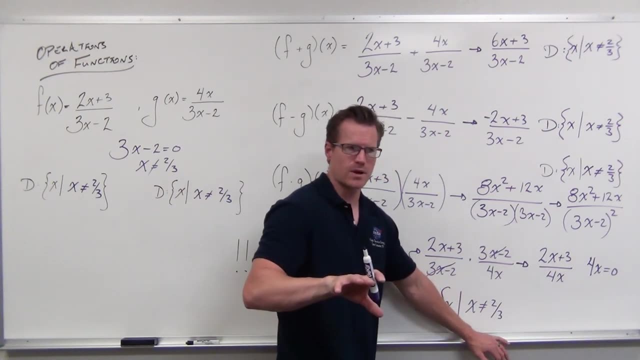 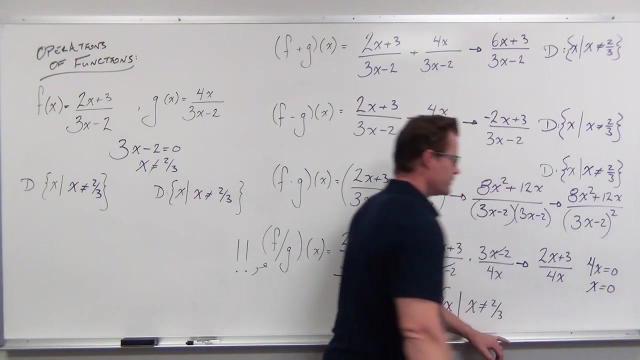 let's find the domain of this. Say, well, 4x equaling zero wouldn't be good Because that creates an undefined issue for an output And we know that the domain needs inputs to give us defined real numbers. And I divide by 4.. Zero divided by 4 is zero. You go okay. 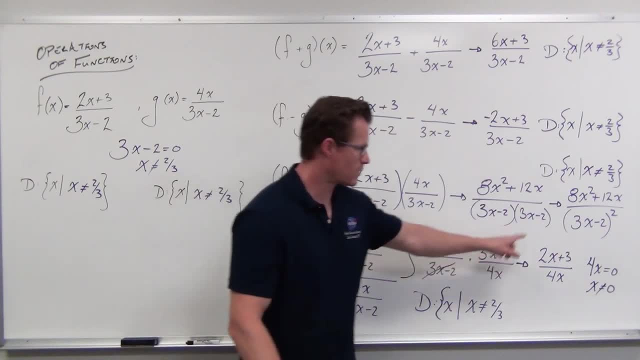 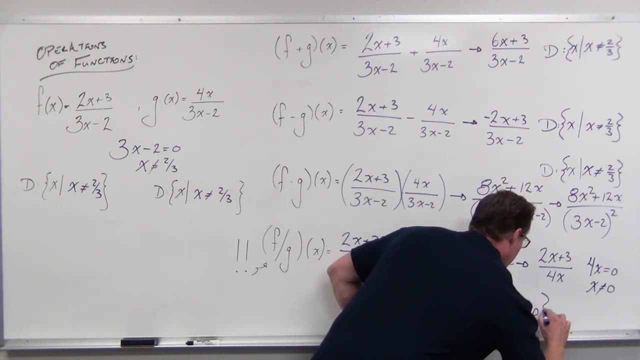 yeah, hey, x equaling zero would be not a great thing. here We'd get 3 over zero. That's undefined, So I know that I'm going to exclude zero. If we ignore this and have that, we do understand domain. 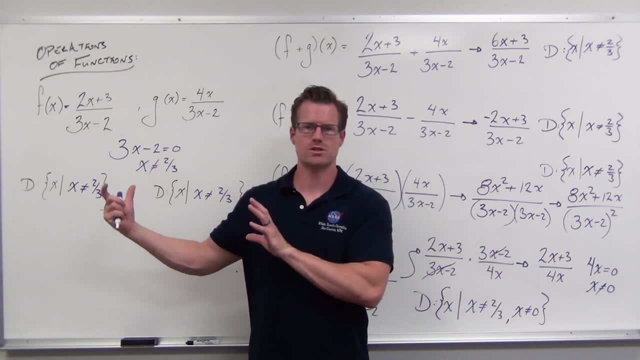 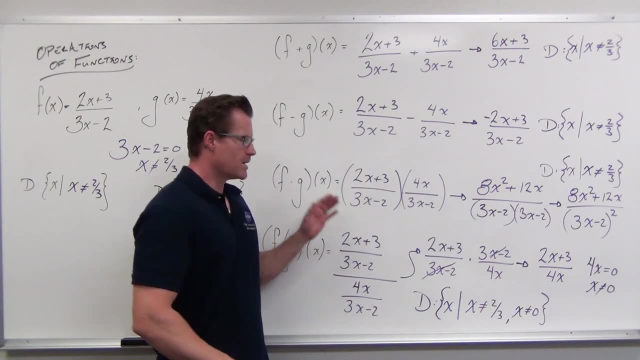 But we're forgetting to realize where the functions came from. So when we go ahead and we do division, how to appropriately approach this is: find the domain first. When you start dividing, make sure that you write that domain down. You go okay, whatever these are you're. 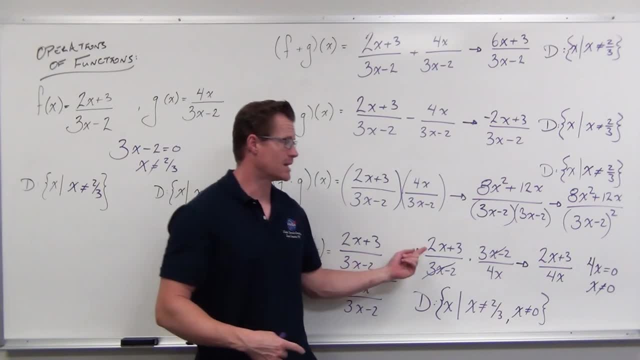 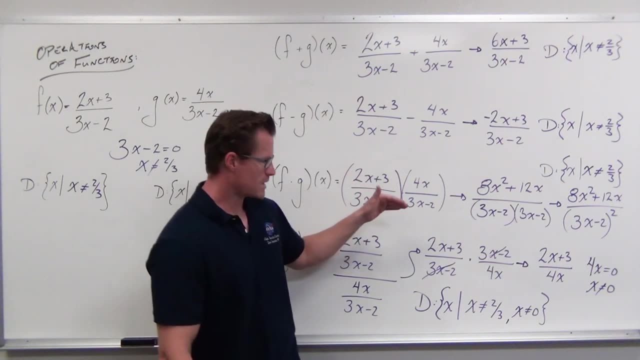 going to have it here no matter what, And then we might even get additional domain restrictions that we have to add to that. We have to exclude that from the domain. So, even though it looks like the 3x minus 2 cancels out, it does, But the domain issue is still there based. 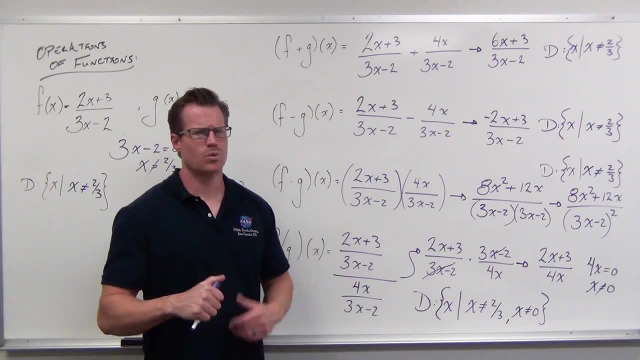 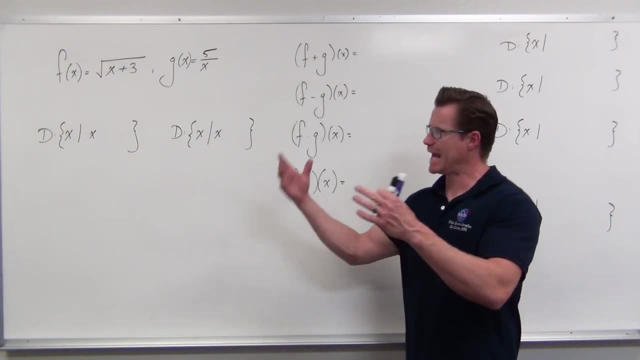 on where we came from. Hope that makes sense. We're going to go ahead and do one more really quick one, just to talk about a square root. You hit that one more time and then we'll be done. Okay, last one. So we're going to add these, subtract these, multiply these and divide. 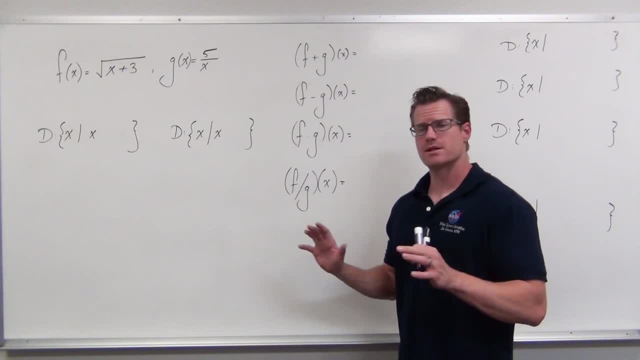 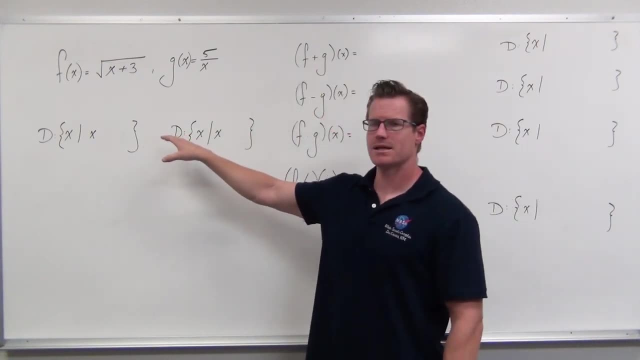 these functions And we're focused on the domain. So really, if you want to stop this and go through here, your first process should be: let's think about it, find your domain first and then recognize that, no matter what I do, I'm going to have these two domains. 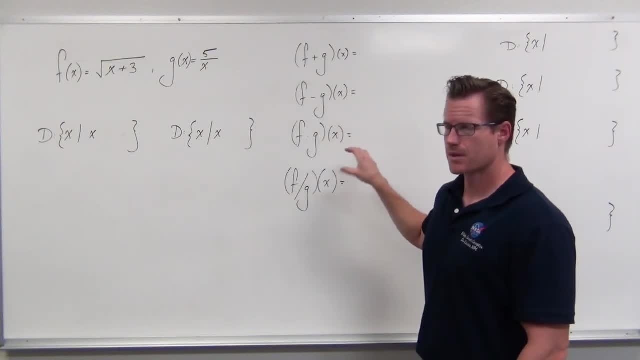 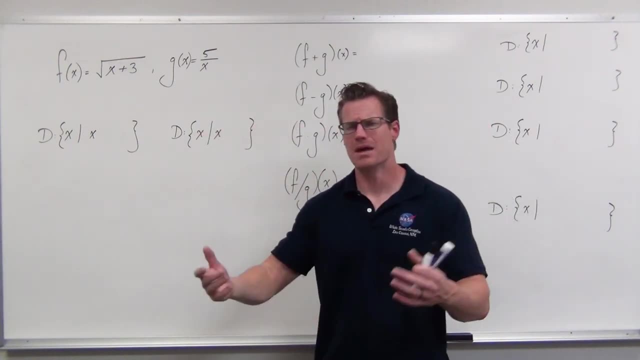 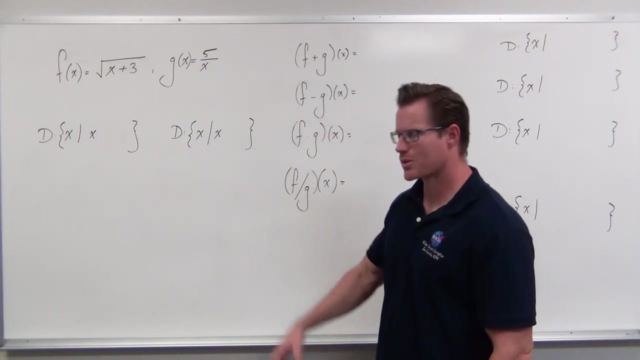 in the result of every single one of these functions, One of these function operators, and I might even add some to it. So I'm going to have at least what's here and maybe add domain problems as we're doing these operations. So let's go ahead, Let's do our domain. Oh man, so we think about it. Last time we were. 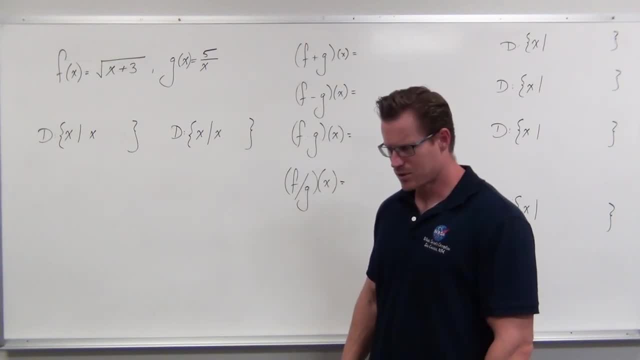 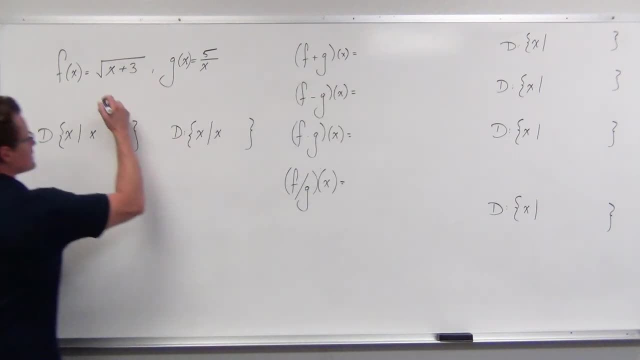 going to think about domain like this for a while. So I look at the square root and I think square roots are this idea that they want to be positive. So it tells you what it wants to be. It says I want this inside this radican to be positive. So I'm going to 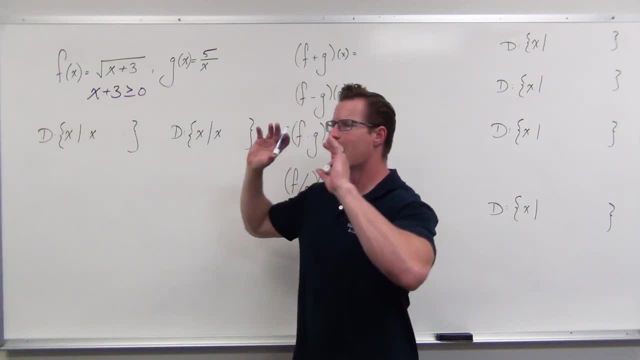 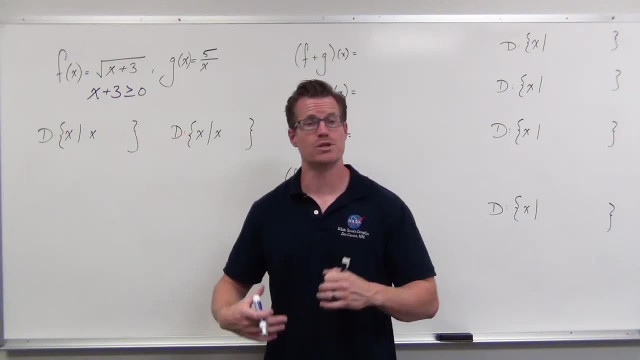 say positive or at least zero. So we think about square roots and say I need real numbers here. What makes it happen? It makes it happen if the inside is greater than or equal to zero. If not, I get imaginary numbers. That's an issue. I subtract three and it says that: 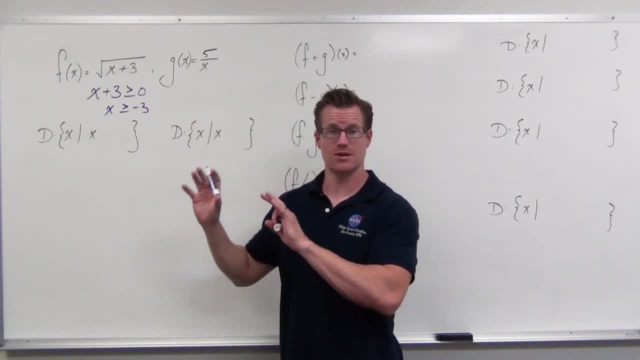 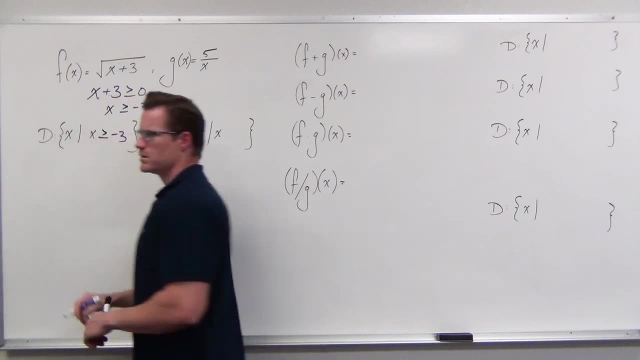 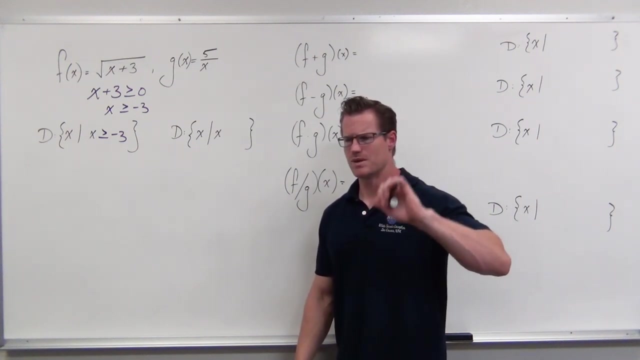 I need x to be greater than or equal to negative three in order for this to give me real numbers out. That is the domain of that function. Then we go to denominators. right here, this function g of x, What about denominators, In order for this input, these inputs, to give me a real number. 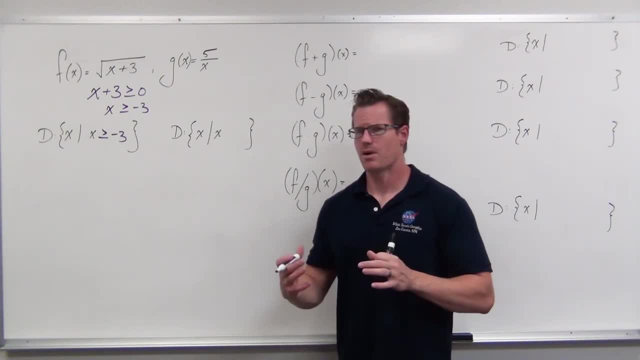 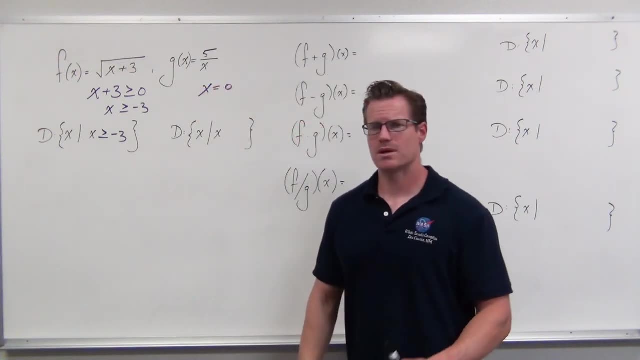 defined value out. Well, it's not about negative or positive, It's about defined values for fractions. We know that if x equals zero, I'm going to have my denominator equal to zero. That's giving me an undefined value. That's going to be a problem. So any positive. 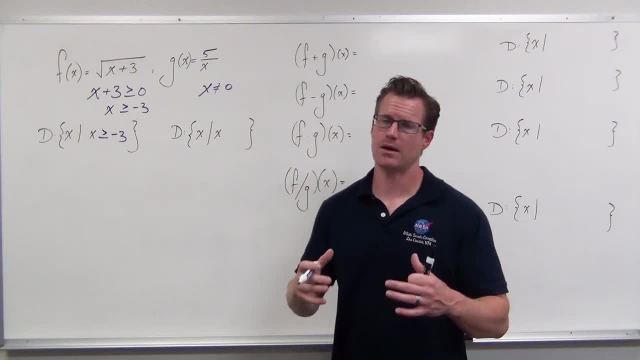 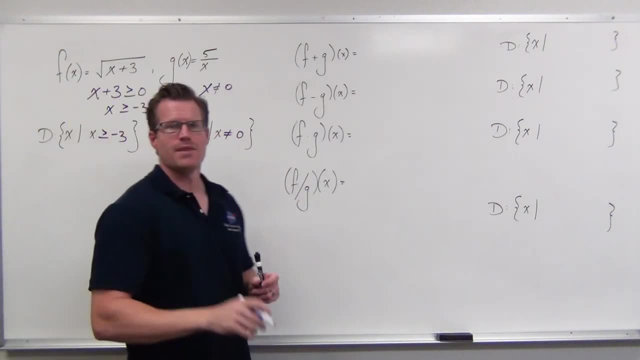 is fine here. Any negative is fine here. But we just cannot allow zero to be an input for that particular function. So we're going to say that, yeah, x equals zero. So we're going to say that x cannot equal zero. That needs to make sense before we go any further. So 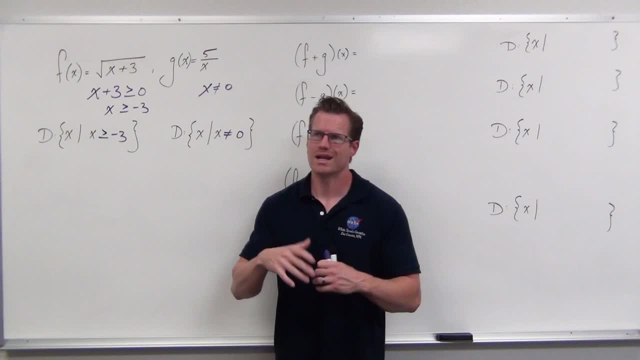 when we look at square roots, we think what's going to give this, or what inputs will make this function? give us real, number, defined outputs For square roots. you've got to keep them positive, solve it and these are the numbers that keep it positive and give you. 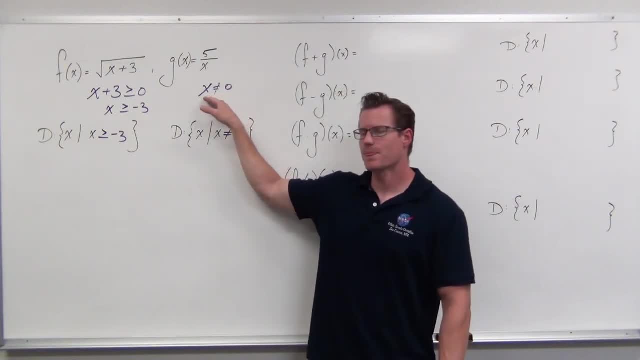 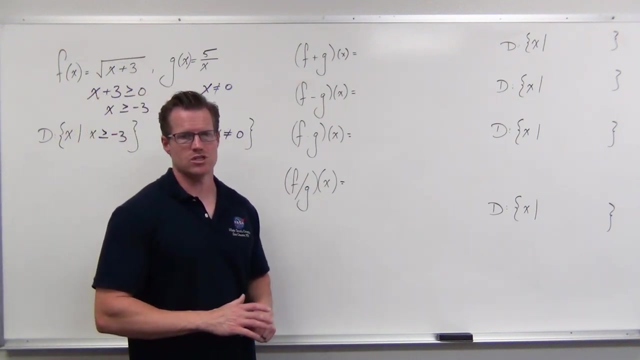 real numbers out For fractions denominators cannot equal zero because if they do, you get an undefined value. So square roots positive denominators can't be zero. These two domains give us for every single one of these, and we might, we might get some more restrictions. 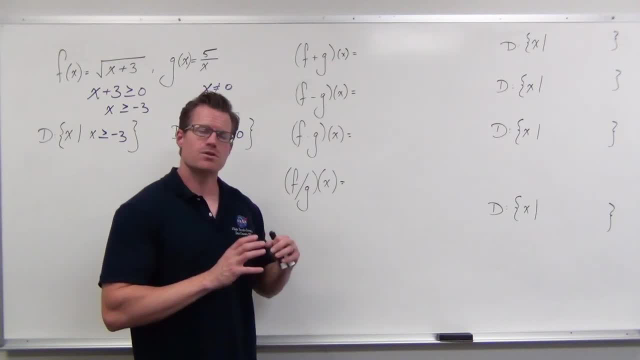 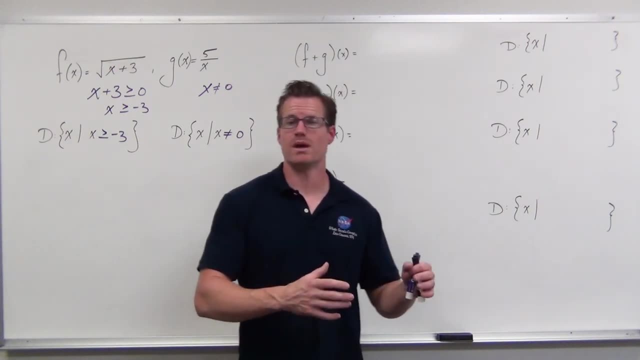 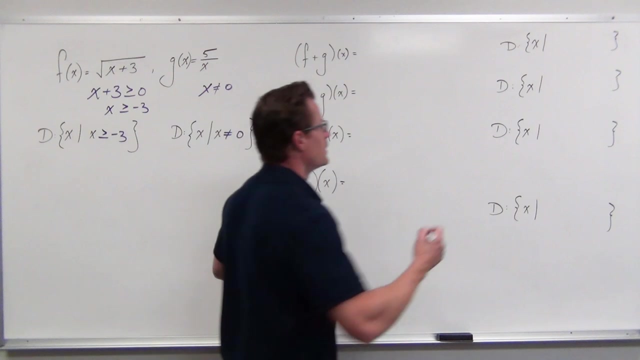 out of it. What can't happen? even if you start canceling stuff out, you are still going to have these. So you never ever cancel away domain restrictions. So if you wanted to do this right now, say, hey, what's my domain? Well, I know that. 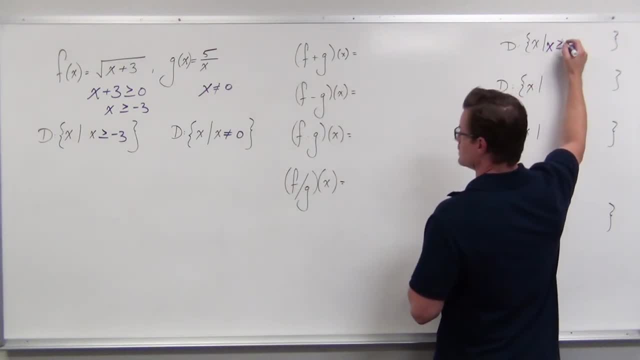 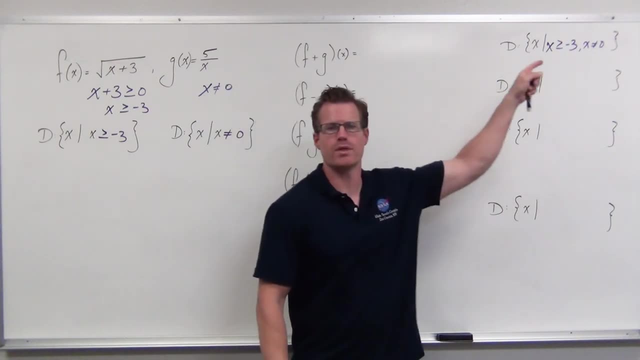 That's got to happen, No matter why I get here. I know that because they never go away. 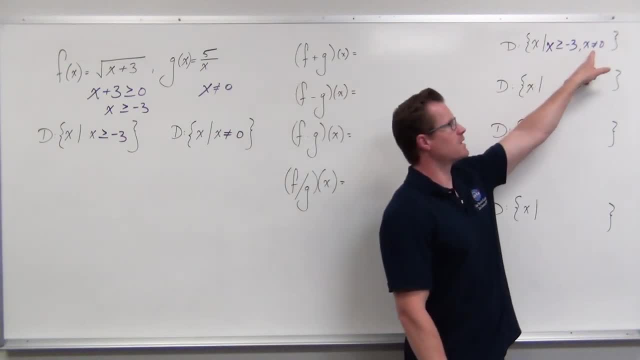 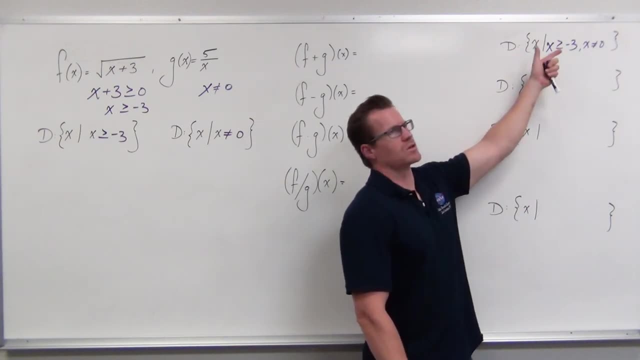 Also, do you, do you realize that this is not relevant here? We had a case last video where we didn't have to put this because it was. it was included in that. Well or sorry, it wasn't included in that interval, Since this says x can be any number bigger than. 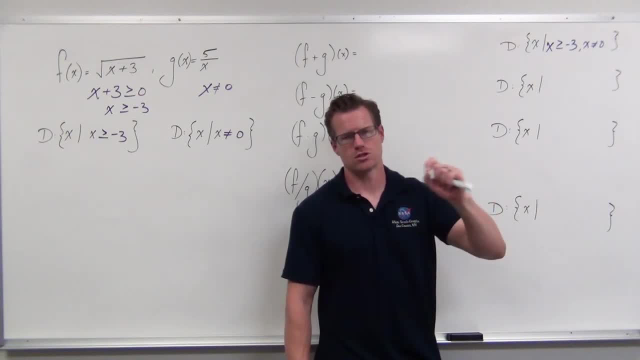 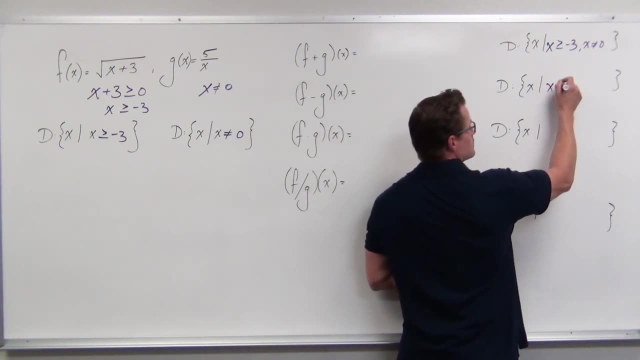 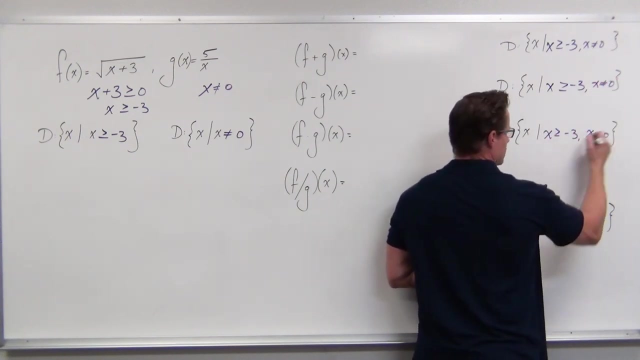 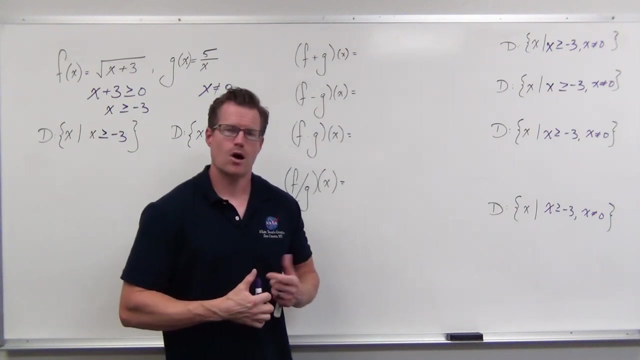 negative three and zero is in that interval. we have to show explicitly that we're excluding it, either this way or with interval notation, which I showed in the last video, Or we can write it here too. same thing, And that might be a really good option for you- to, before even doing this, write down the domain. 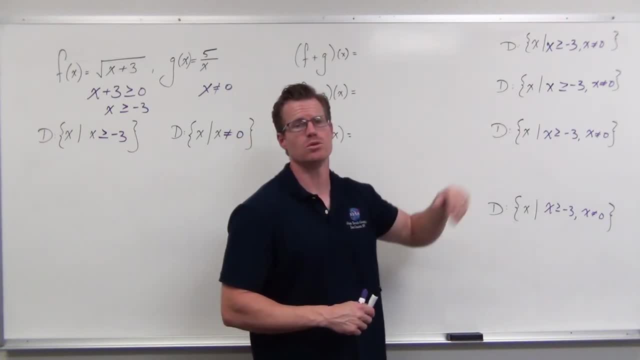 It's not going to change. The only thing is you might have to add some more to it. That could be the case. Well, let's go through adding, subtracting, multiplying, dividing- The first thing. we're going to go very quickly. 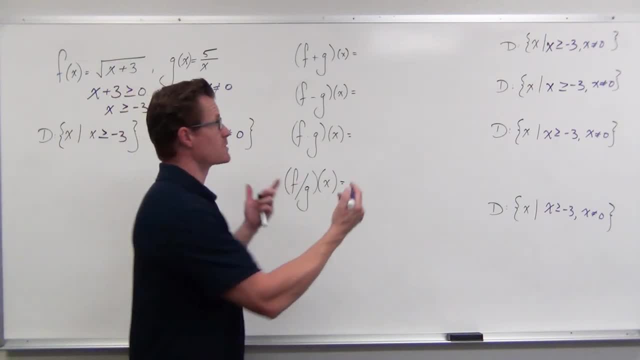 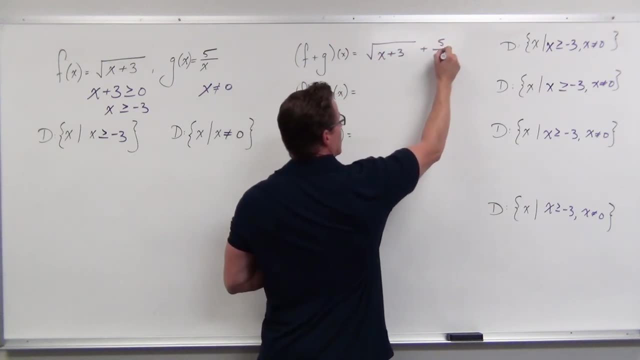 So if we add these functions, there's nothing to really combine. So adding functions says: hey, you're just going to have that x plus 3.. You're going to add 5 over x. And it's very clear to see that that's still the same exact domain. 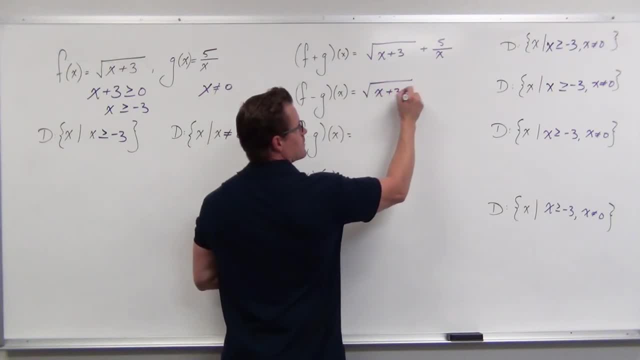 Or if you subtract them, same thing, x plus 3 minus 5 over x, same exact domain, Or multiply them. I'd probably put the 5x first because multiplication is commutative. We can do that: 5 over x. 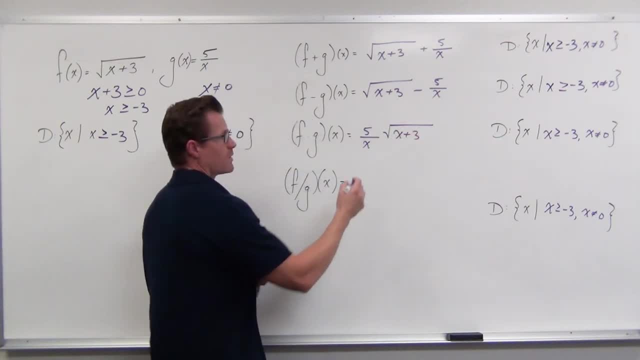 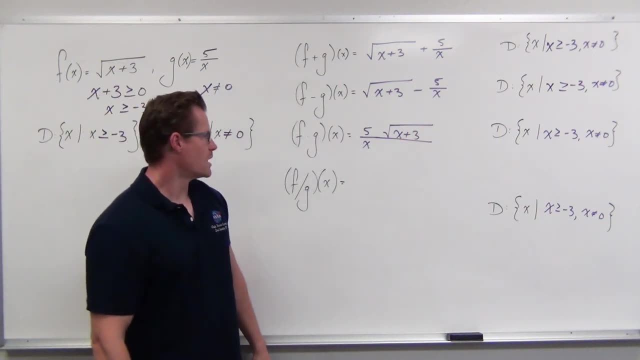 Times x plus 3.. You can even make it one fraction, 5 times square root of x plus 3 over x, And you see that we have the same exact domain. It's not going to change. Now the division. We do have to be conscious of what's coming first, because division is not commutative. 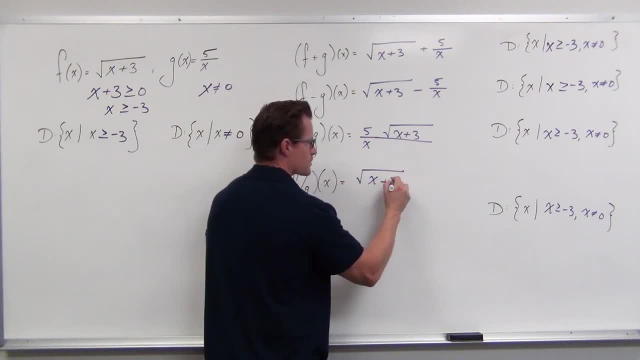 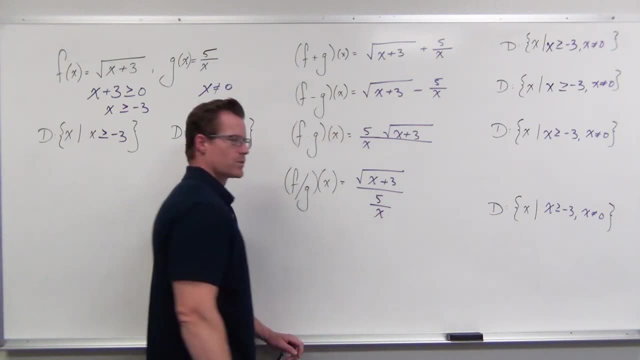 So we'd have to put the square root of x plus 3 on our numerator And we'd have to have 5 over x on the denominator. Well, wait a minute. When we're dividing fractions, we multiply. We multiply by the reciprocal. 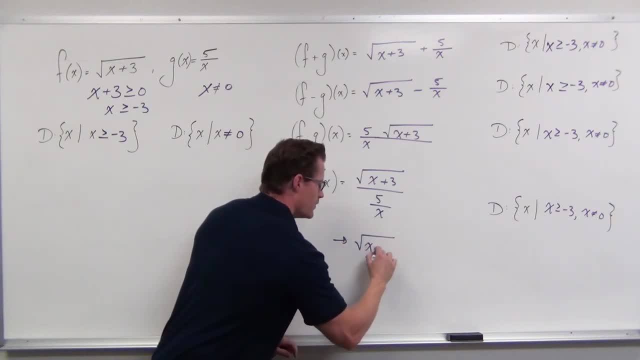 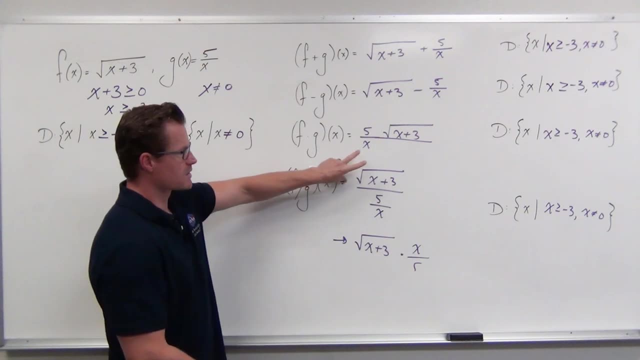 So this would be the same thing as the square root of x plus 3 times x over 5. Times the reciprocal of 5 over x. So here's x. You can think about square root of x plus 3 over 1.. 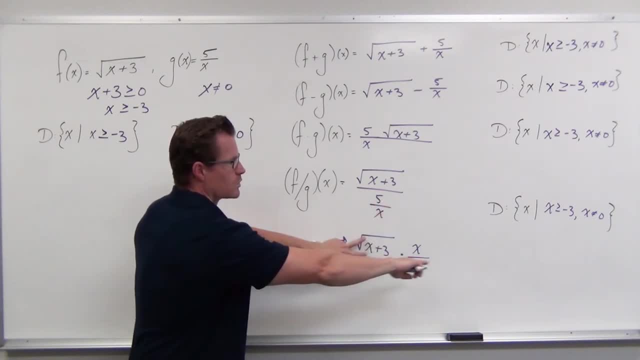 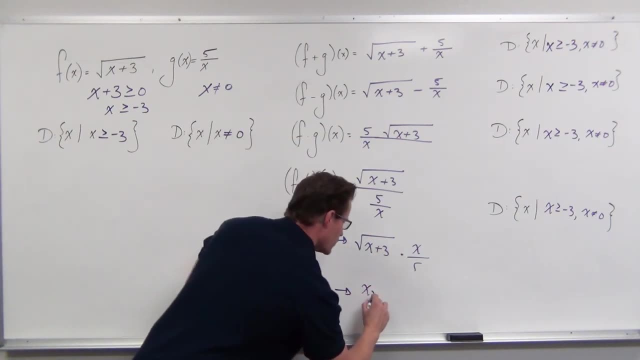 So square root of x plus 3 over 1. Divided by 5 over x. So multiply it by x over 5. You go. this is fantastic. I can simplify this just a little bit. Maybe put my x before that square root. 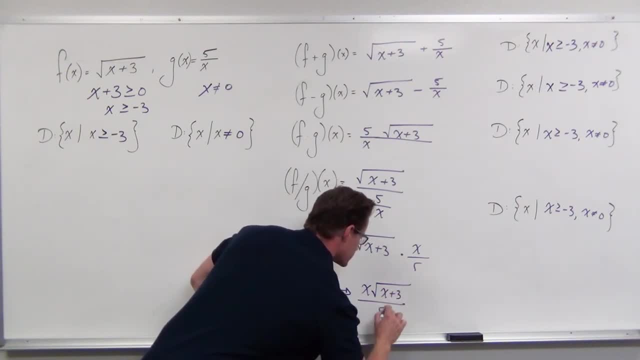 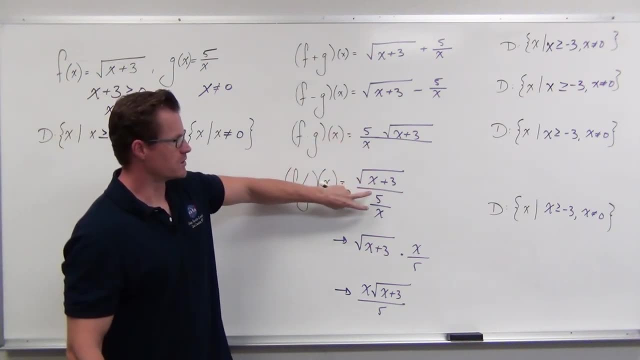 Okay, Okay, Okay, Okay, Okay Okay. That's the resultant function of dividing f by g. We divided square root by a fraction. When you divide fractions, you can multiply by the reciprocal, No problem. We would have x times square root of x plus 3.. 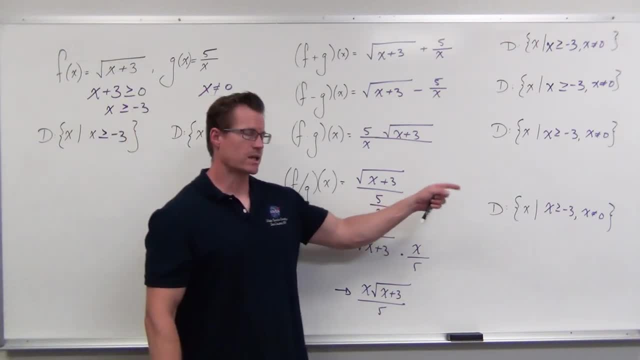 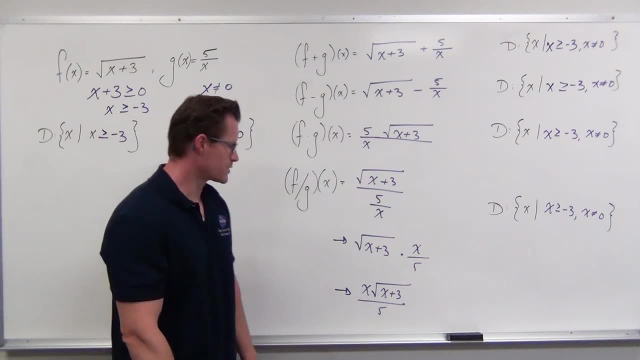 We'd have over 5.. This is one of the reasons why that might be a really good option for you to do first. Do you see it? Do you see how the denominator changed for us? The denominator said: well, there's no longer an x there. 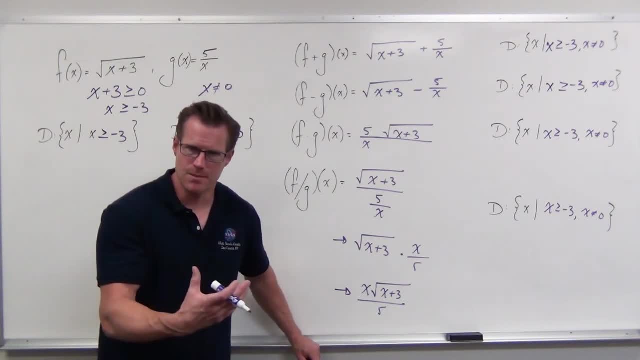 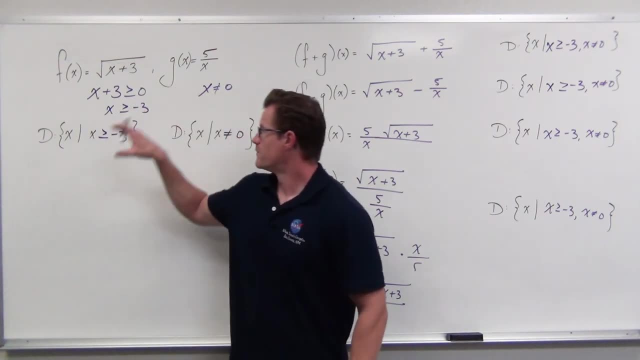 So if you were to just do this and then think about the domain, you're probably going to miss that. Don't miss that. This is why the technique I'm giving you works really, really well. Find the domains first. If you want to write them down for every operation, do that. 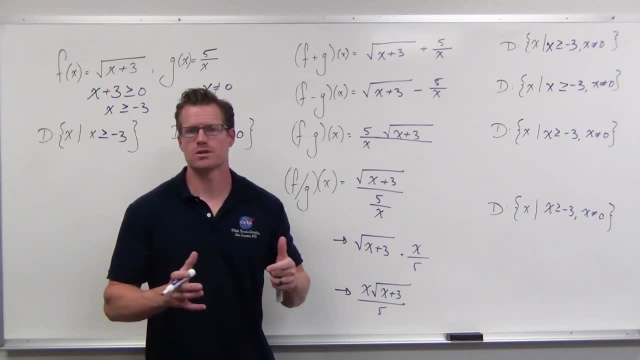 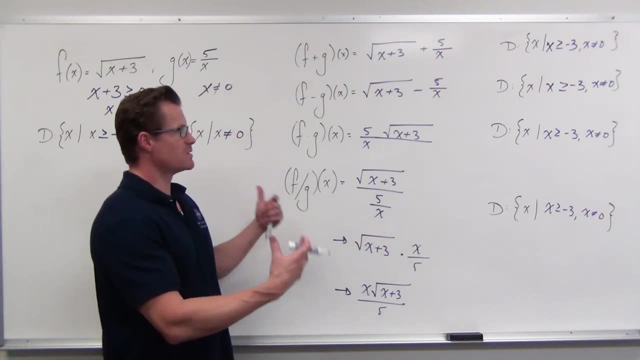 Even for compositions that sort of works Really. we take the domain of the inside function and the final function, So we combine it that way. But for adding, subtracting, multiplying, dividing, you're always going to get the same domain. 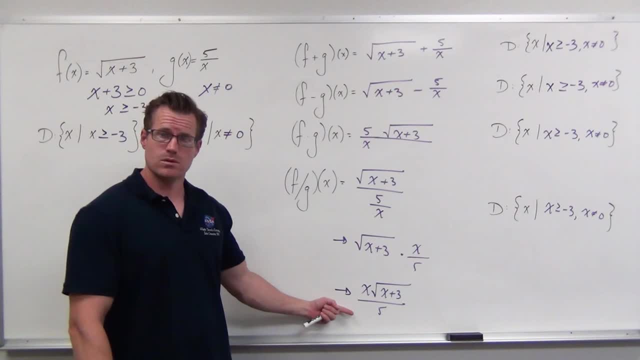 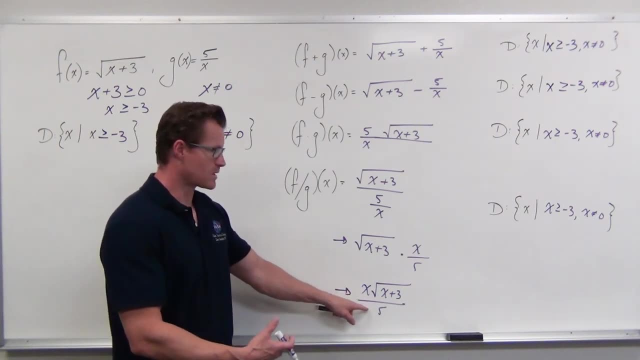 No matter what, because we started with that. We don't add anything new, huh? Because look at that, The square root. It hasn't changed, So that's still the same domain that we had. The x is gone. It looks like that's gone. 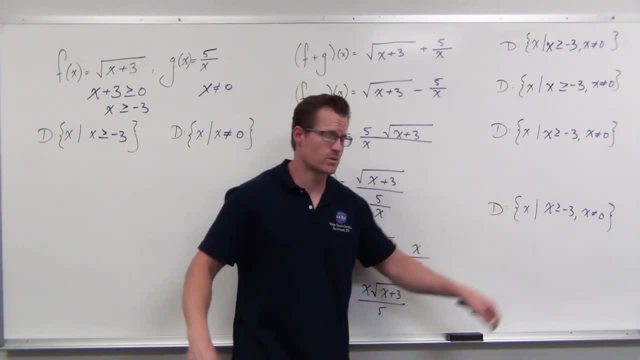 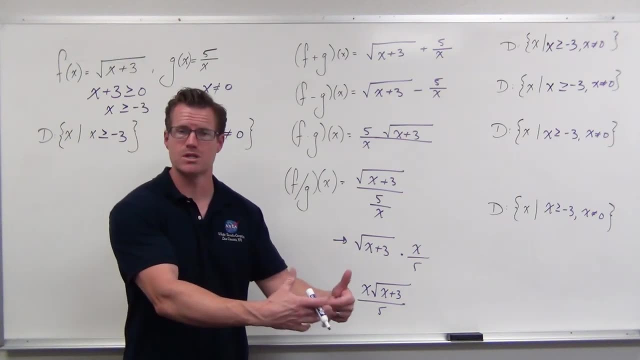 The problem for x equals 0 is gone, But because of where it came from, we have to retain it. But our denominator cannot equal 0 anymore. That right there can't equal 0. So we don't gain any new problems. 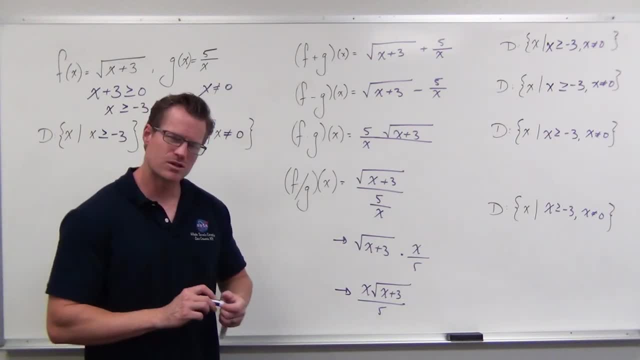 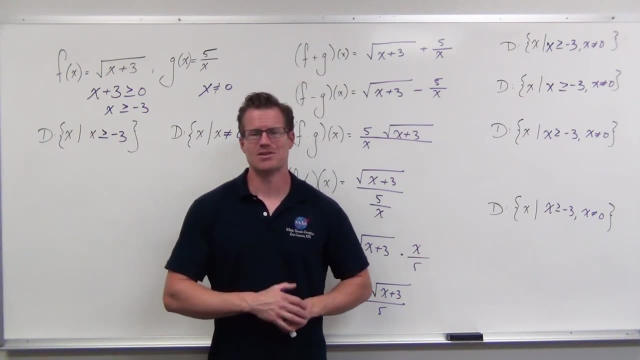 You still have the same old ones. I hope that makes sense. I hope you understand at this point that your domain does not change from your original functions when you're doing these operators. You can only kind of make it worse if you divide, So practice that. 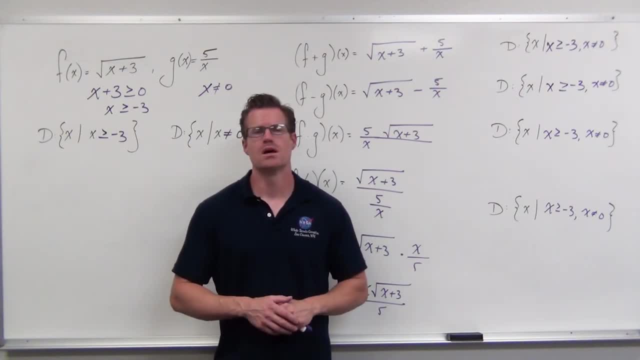 I hope that makes sense. Next time we're going to talk about some graphs of functions, determining if one input has to give you one output. what that looks like graphically. So we'll do something called the vertical line test. You've probably heard about it, but we'll explore why it makes sense. 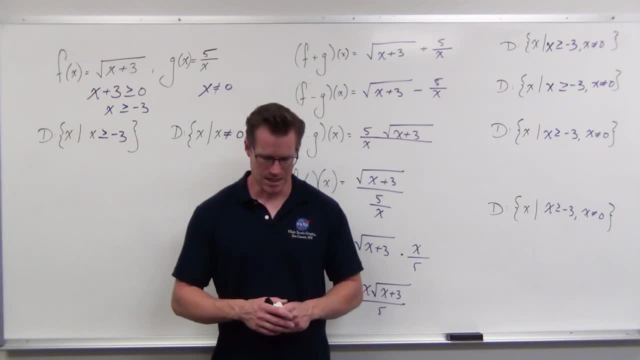 We'll talk about even versus, odd functions and some more things like that. So have a great day and I hope to see you in the next video. Bye.